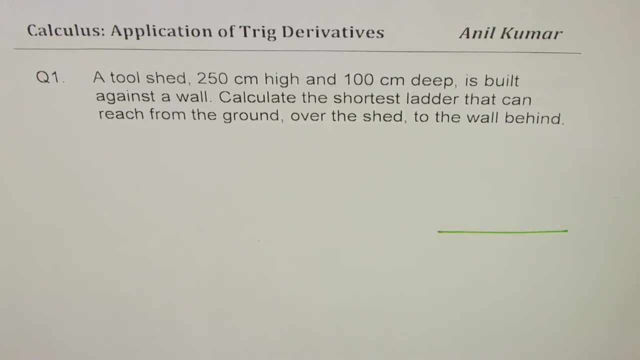 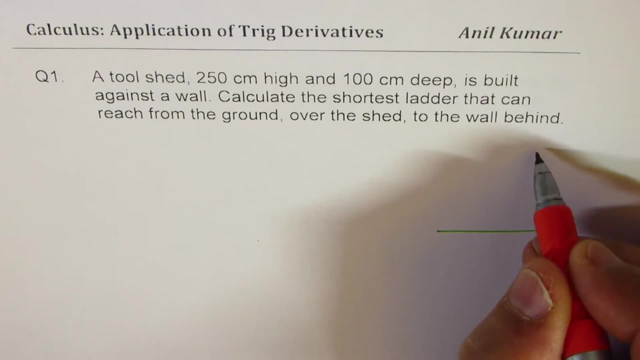 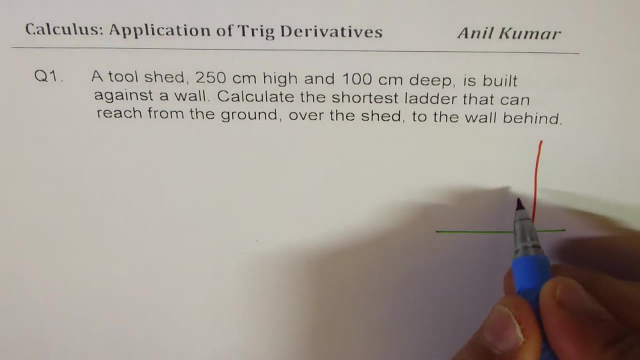 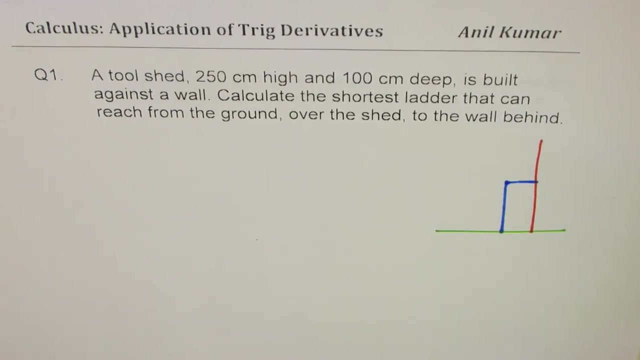 sketch the diagram right. So we have a tool shed which is 2 centimeter high and 100 centimeter deep and is built against a wall. So let's say this is the wall for us, right? And the shed is kind of like this: A ladder leans against this shed, So let's say the ladder could be. 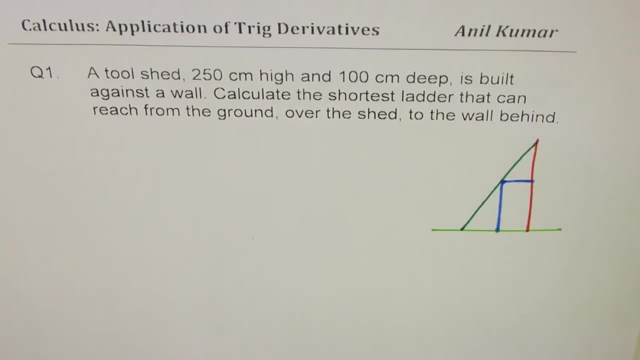 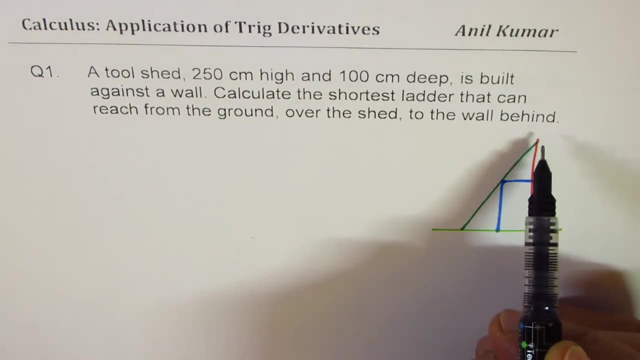 let's position the ladder like this. In that case we need to calculate the shortest ladder that can reach from ground to the wall right. So that is the length L, for example, for the ladder. We know this is 100 and this length is 250 here, all in centimeters. 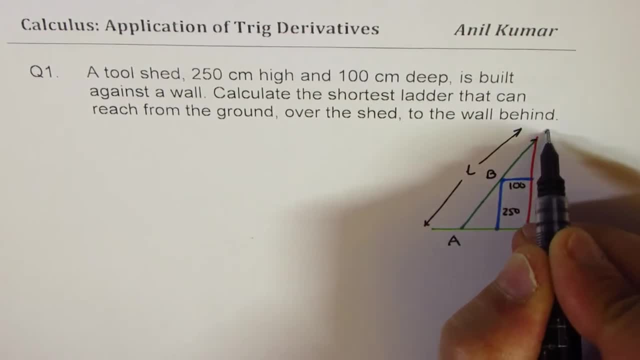 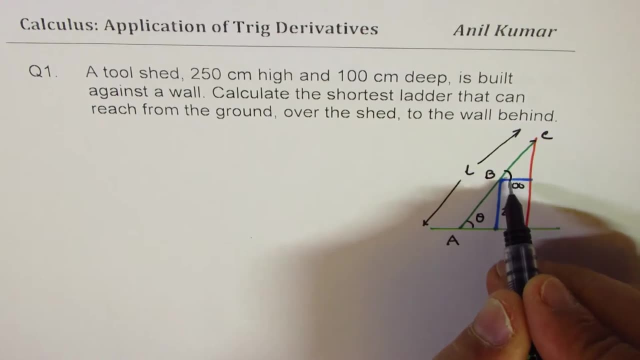 Let's say: this is point A, this is point B and this is point C. Now the angle here will be same as angle at B. That is very clear, right? So let us say that the length of the edge of the head is 50 or 300 millimeters. Then the degree of angle looks the same as the degree of angle at the base of the head. So that is very clear. But actually the angle here is it'sars and it could be anywhere around 3 centimeters. Yeah, so we'll just try to find out the same as the angle at the base of the head. 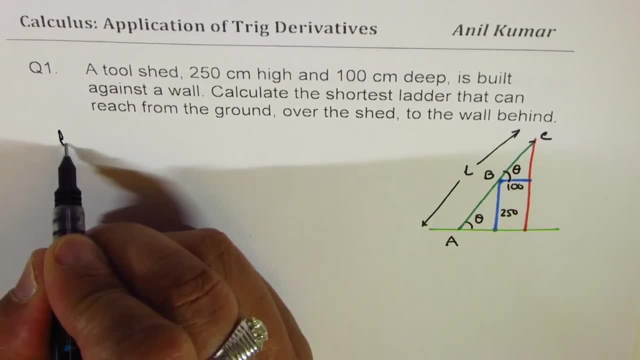 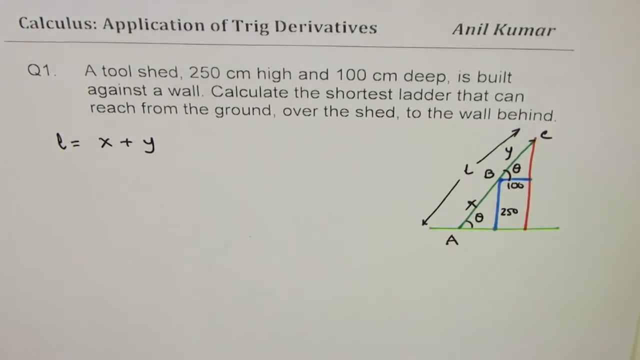 And let's push x and x- Because Z is minus 3 rotations together- for this piece of H to the t series of f and for some T, the letter is X plus Y, where X is AB and Y is BC. in that case we can write both. 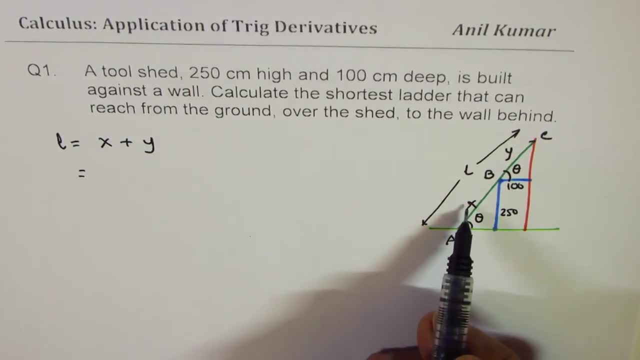 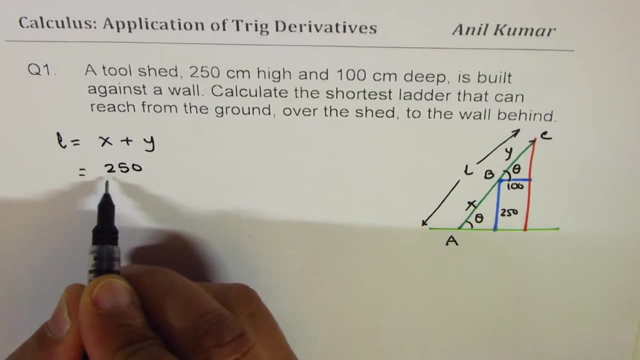 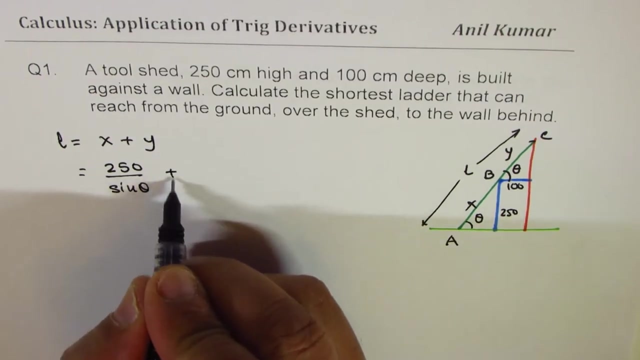 X and Y in terms of theta, and X can be written as: with relation to 250. we can write X as 250 divided by sine theta right, since sine theta is ratio of a positive or hypotenuse. similarly, we can write Y as a ratio of adjacent side. 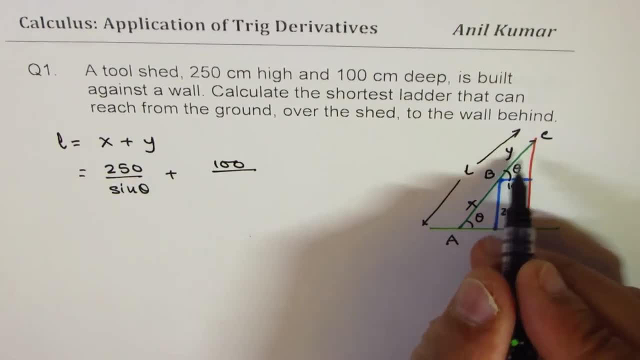 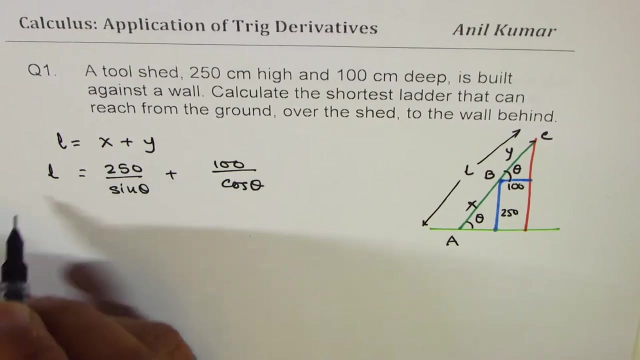 hundred over hypotenuse, so that becomes Y, becomes hundred over cost it. hypotenuse is always greater and sine and cosine are less than one. so it makes sense right now, once we know that we can actually to find the shortest length of the ladder, we can find the derivative. 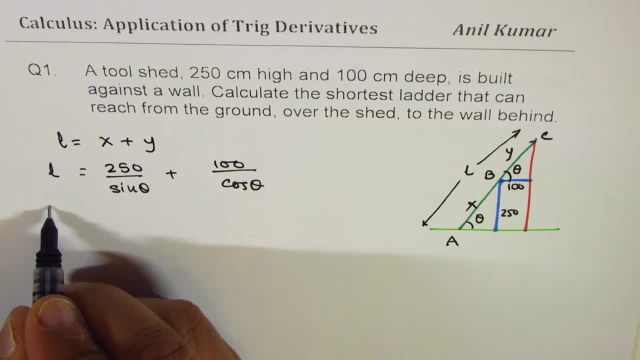 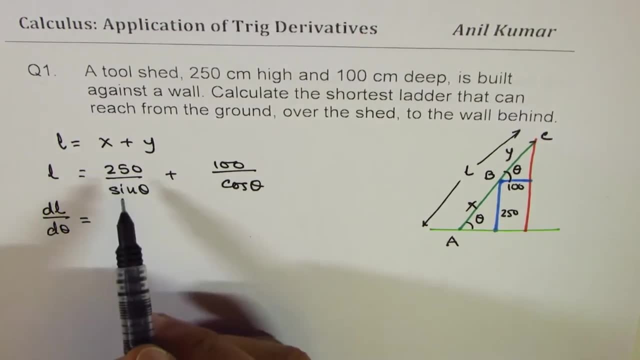 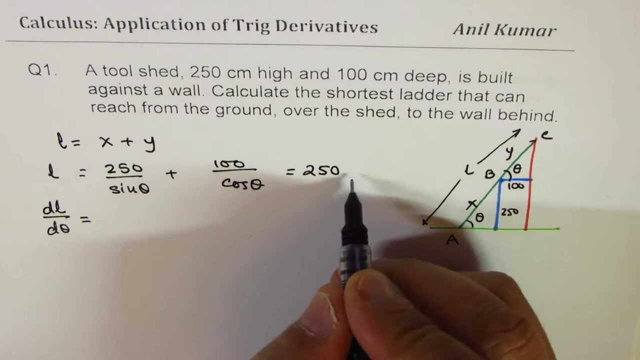 of this with respect to else, to with respect to theta. so DL D theta is equals to derivative of this. you can actually write this as cosecant theta and then do the derivative, or you could do direct also, right. so think like this: we have 250 sine theta, minus one thing like this: 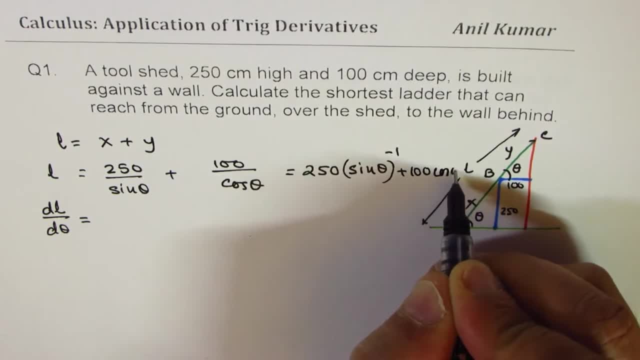 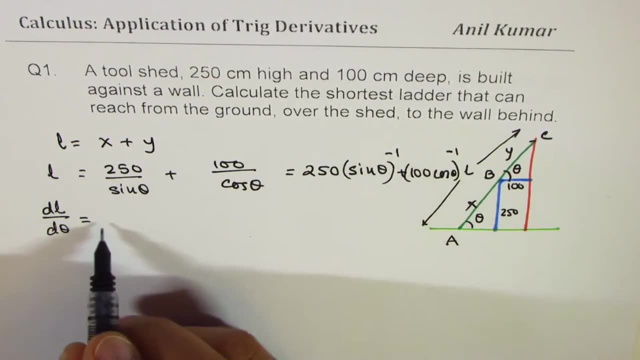 plus a hundred Gauss theta to the power of minus one. so it becomes simpler. you can apply the power rule, is it okay? so that gives you minus of 250. so we are avoiding the formula of cosecant and secant, since you may not remember it, minus sign theta to the power of minus two, so that becomes minus two times. 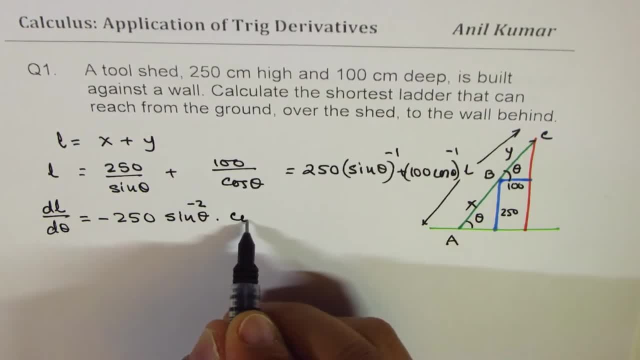 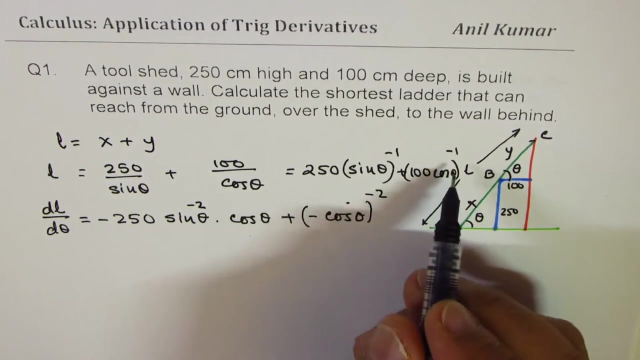 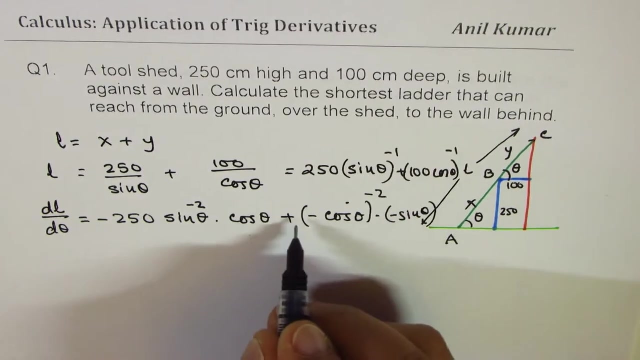 derivative of sine theta, which is cos theta. does it make sense? right, so you could get like this: plus, here again minus. we get derivative as minus of cos squared cos theta to the power of minus 2 right times derivative of cos theta, which is minus sine theta. does it make sense? and of course I forgot to write. 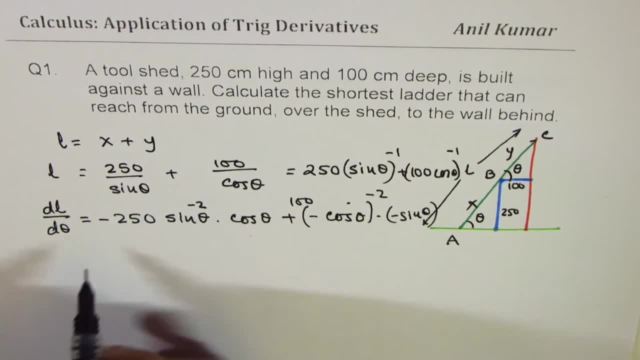 hundred, is it okay? so you go right like this. in a way, what you get here is minus 250, cos theta divided by sine squared theta. plus and minus becomes minus, and that minus makes it positive. so here we have hundred sine theta in the numerator divided by cos squared theta is that? 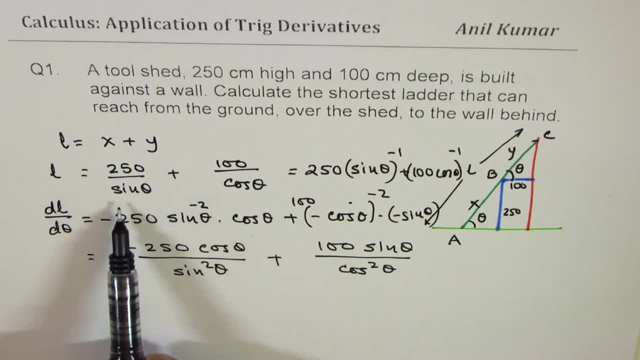 here. well, you could have written directly derivative of cosecant theta and secant theta also. okay, now for maximum or minimum, which we say critical number DL. the theta should be 0, so we can equate this 2 to 0 and then find the value. is it clear? so, multiplying by: 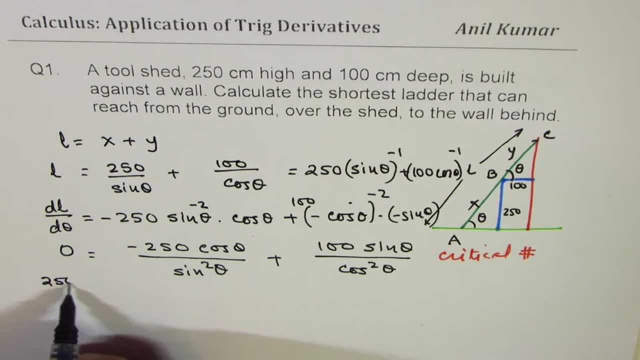 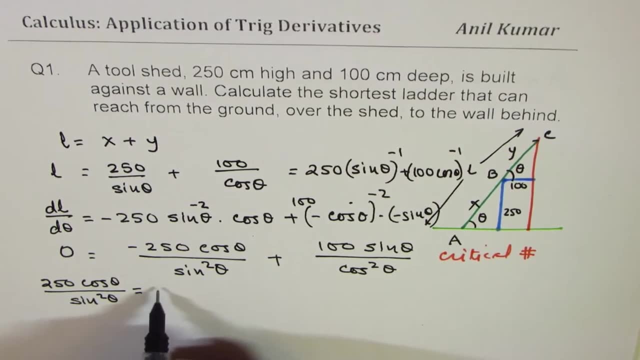 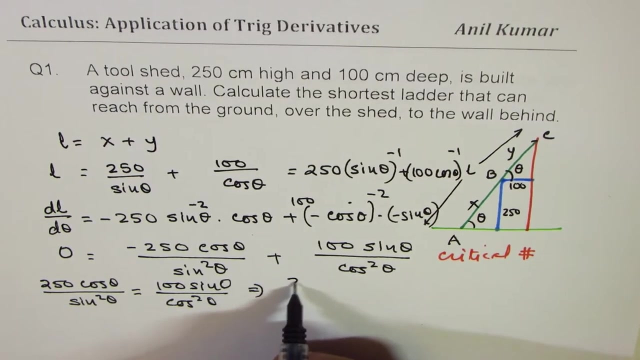 or we can just take this side to the other side. we get 250 cos theta divided by sine square theta equals to 100 sine theta divided by cos square theta. now, if you cross multiply. so what we get here is that gives you 250 over 100 equals to 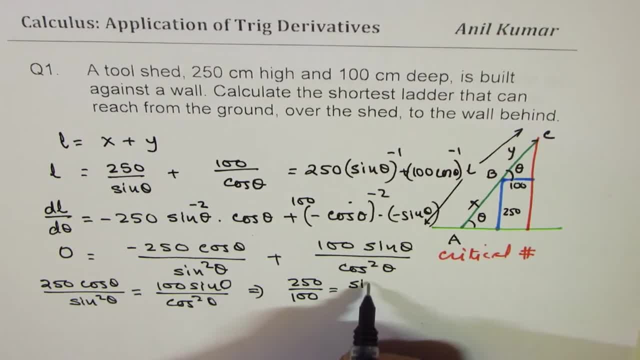 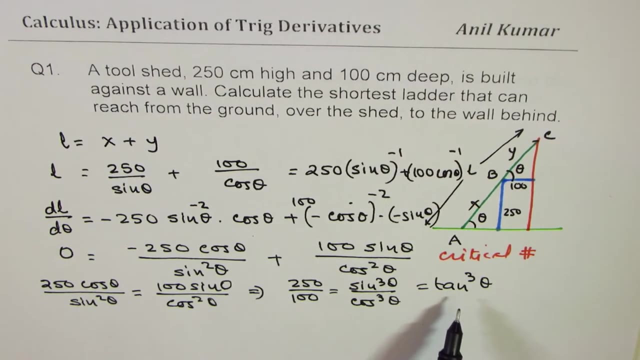 if you cross multiply, get sine cube theta divided by cos cube theta correct, which is tan cube theta, right? so we know tan cube theta is 250 by 100. so from here we can find what theta is. now the angle theta is actually between 0 to 90. 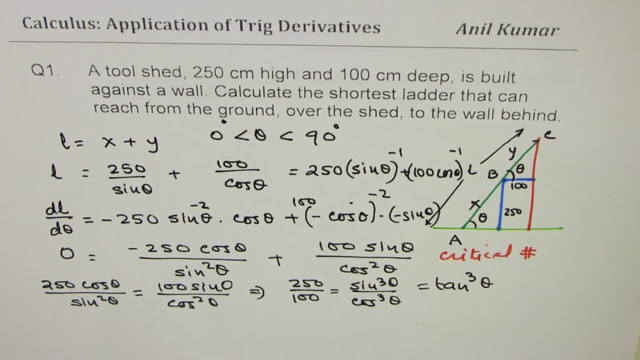 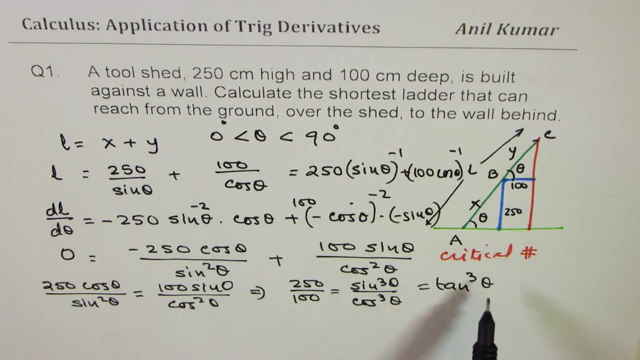 degrees right to form a triangle in this figure fashion. now we we know that somewhere in between we will get the minimum height, since when theta is approaching 0, when theta is approaching 0, in that case 250 by sine. theta approaches infinity right, so this becomes infinitely large. but when 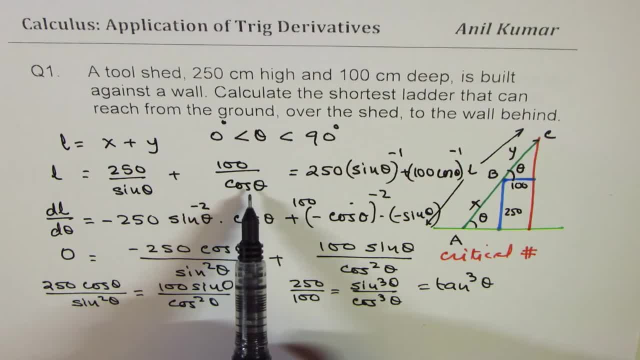 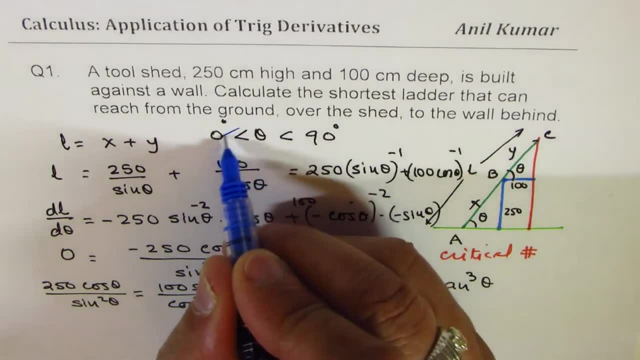 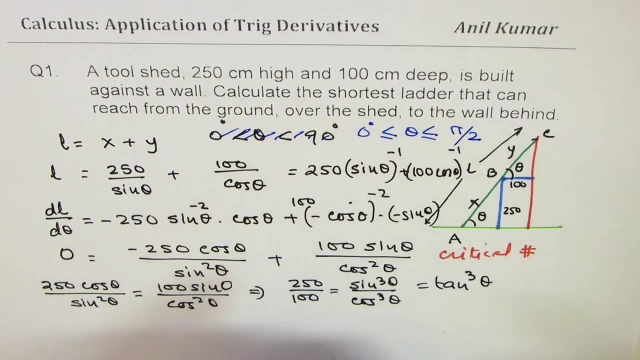 theta approaches 90 degrees, cos theta approaches infinity, right? so time is 10 times the number of degrees, and that number is actually 10 times the answer for this number, right? well, when we are working with the trigonometry, we should actually do it in radians. so we'll write this: 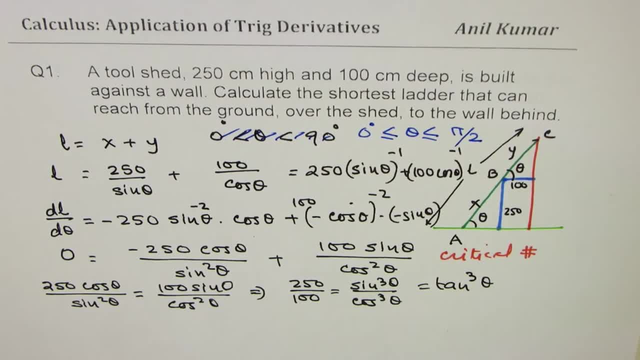 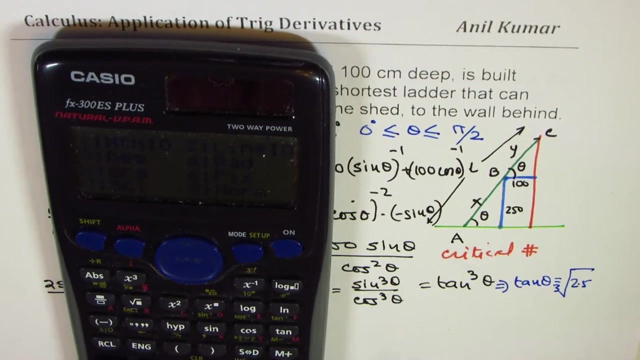 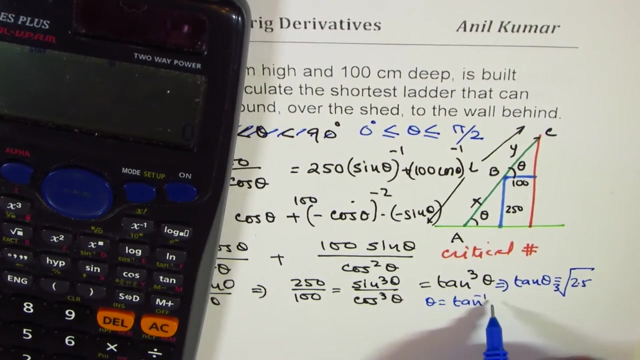 from 0 to pi by 2, is it ok? so anywhere in between we are going to get minimum right now equals to cube root of 2.5. right, and let's convert our calculator to radians, so we get 4. so that gives you radians. now theta is equals to tan inverse of cube root of 2.5. is that clear? 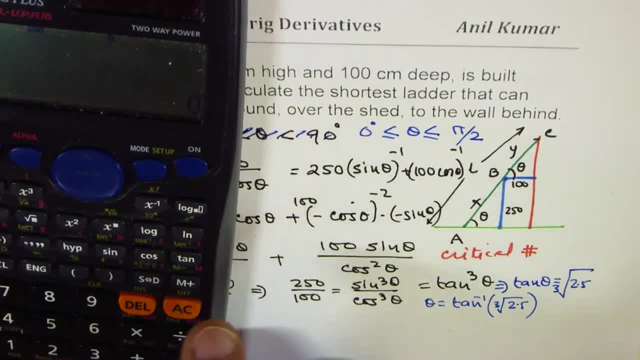 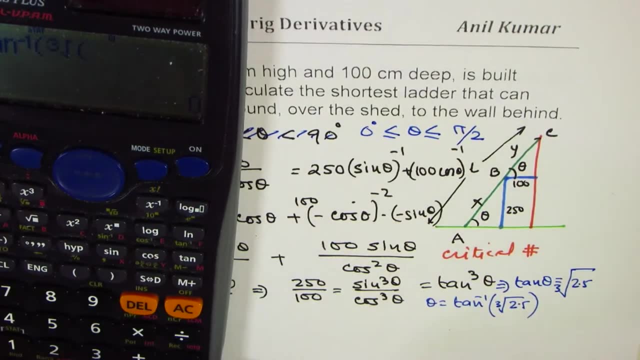 okay, let's do it. so we have shift tan inverse of cube root of. so that is, cube root of 2.5, which is equal to in radians, theta is equals to 0.93579. okay, whatever. so that gives you the value of theta now. 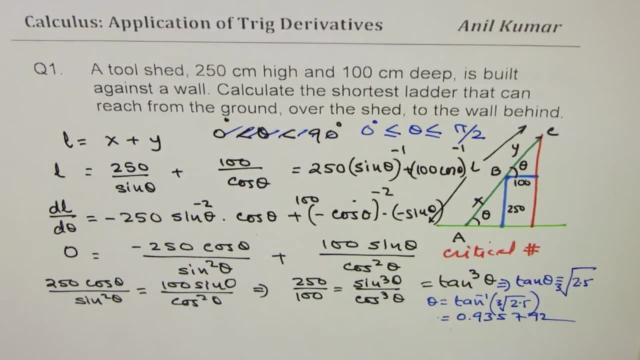 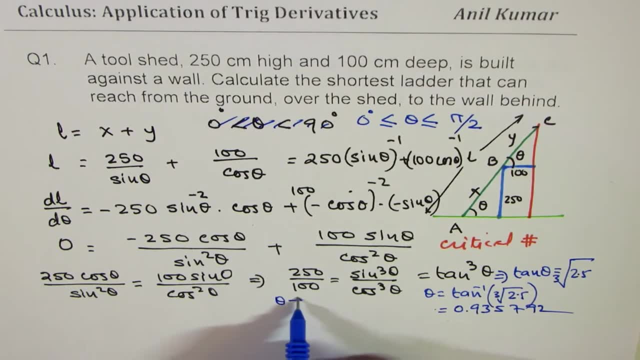 for this value of theta, we can find what l is right, so let me push this page a bit. okay, now we know this is minimum, since when theta approaches approaches 0, from the positive side l approaches infinity right, since sine, theta approaches 0 when theta approaches 90 degrees. 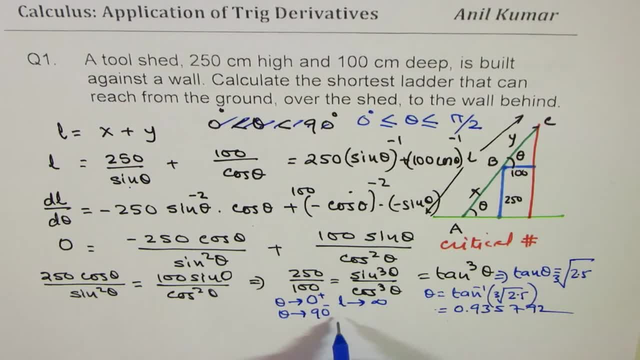 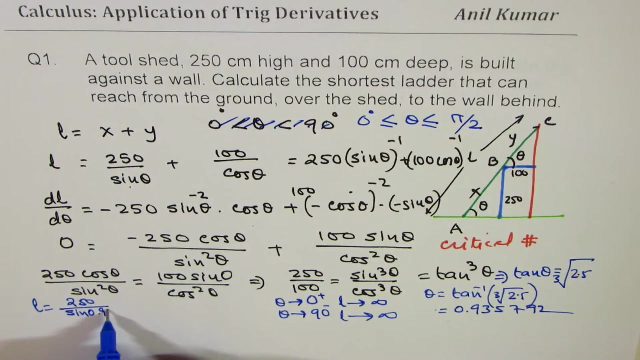 let's say minus. right, it cannot be 90. in that case the length again approaches infinity, because cos theta approaches 0. do you see that part? so therefore anything in between is minimum, right? so the minimum length l will be equals to 250 divided by sine of 0.9. let's say 358. 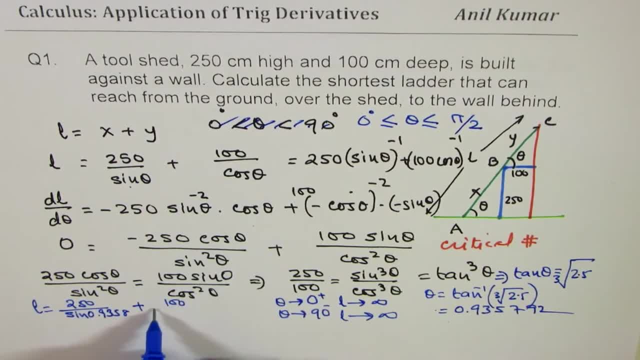 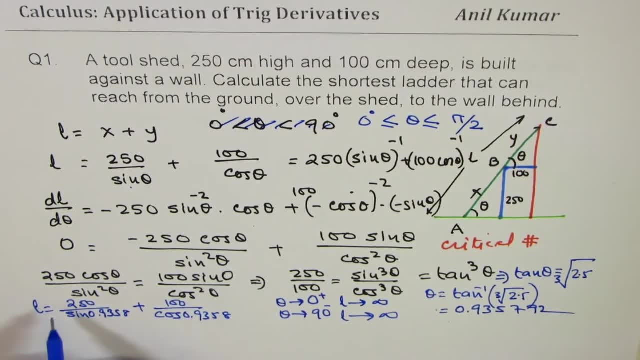 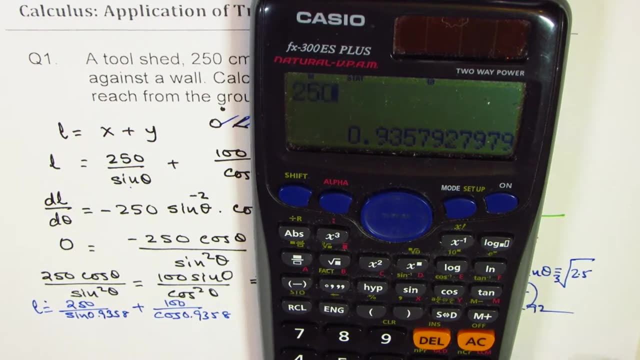 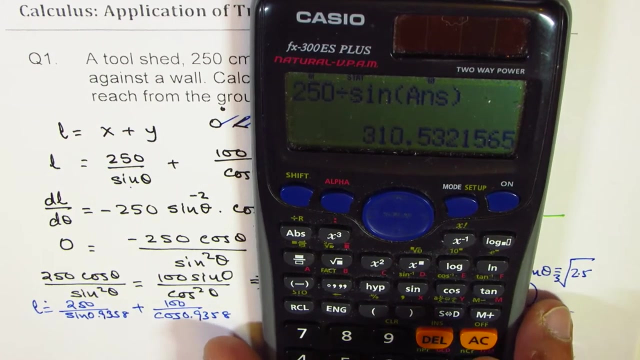 plus 100 divided by cos of 0.93, let's say 5, u1. is it okay? we'll approximate. let's approximate this answer. so what we get here is we already have, for i we can say: 250 divided by sine of our answer, we get three hundred ten point five. so so this is three hundred. 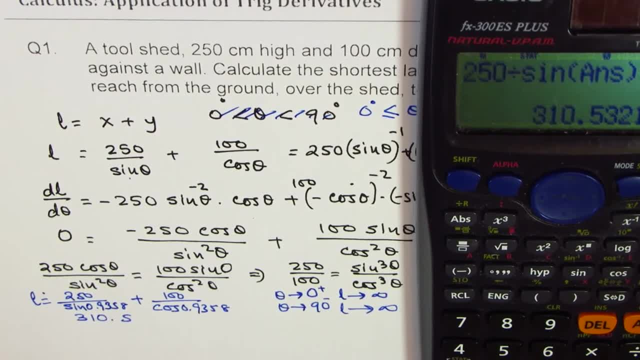 and ten point five. let's push this plus hundred divided by cos of 0.★5 of capital plus value of promotions as pita s, and we can just use this only z, so von wes凩 of sigma for, and we've got exactly the same problem here. let's calculate that we now know that this f m evat x, if I. 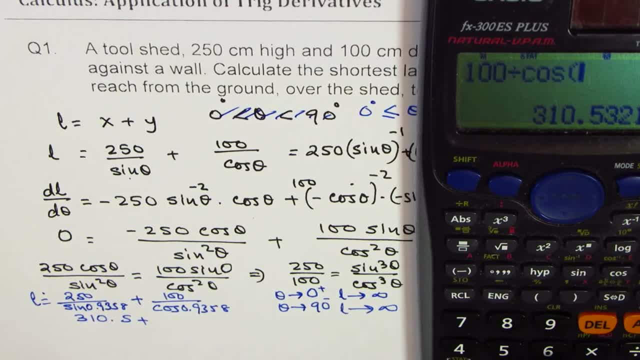 wanted to say in Counsel's. in our case x is the v, meaning f, and next we just change the case variable phi to omega, as follows: so all the parameters are空ieren and we won't be able to kind of define this f and so on. so this one word we'll fifty and all the差 we need to do so f, function f, because if what we're 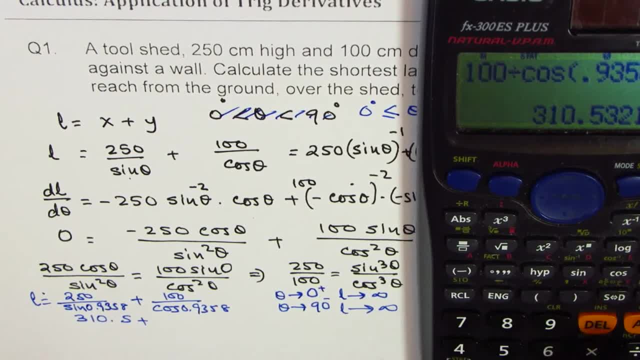 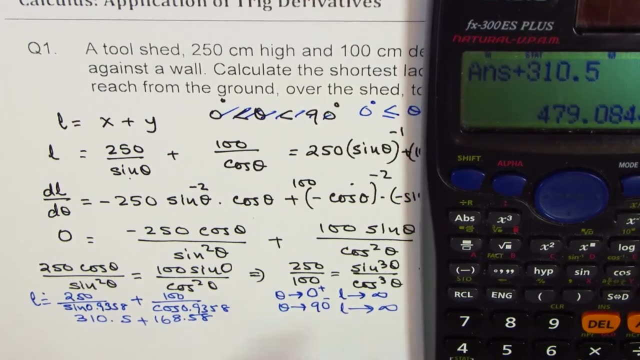 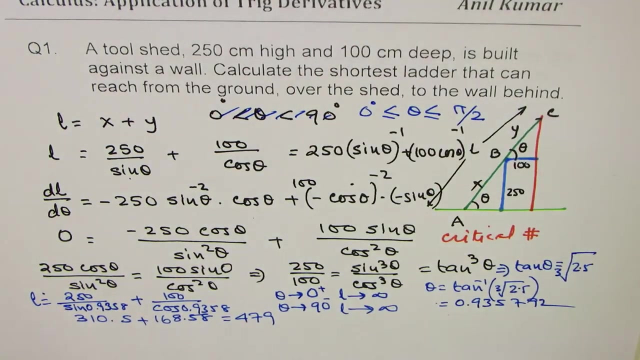 point nine. three five, eight equals to one sixty eight point five, eight. let's add them. so this much plus three hundred and ten point five gives you four point seven, nine. I mean four, seventy nine. so it gives you four seventy nine, right, okay? so what we get here is 479 centimeters, which is approximately four. 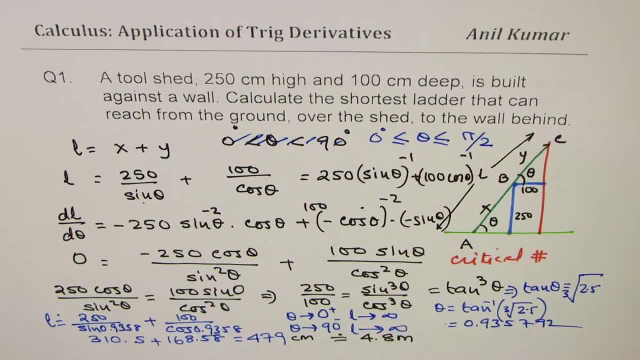 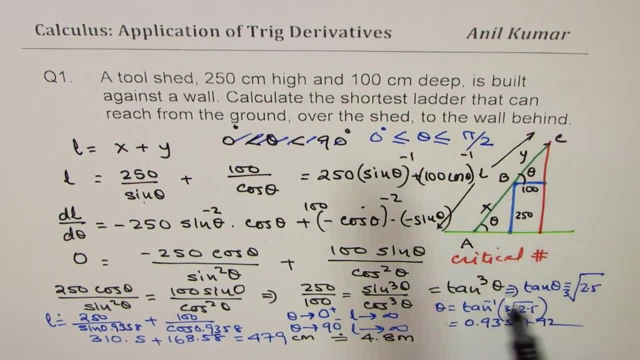 point eight meters. I hope the solution is absolutely clear. let us review. we actually wrote length of the ladder as X plus Y. X is 250 related with 250 divided by sine. theta: Y is hundred divided by cos. theta took the derivative, found the critical number, equated that to zero and then figured out that the angle in radians is: 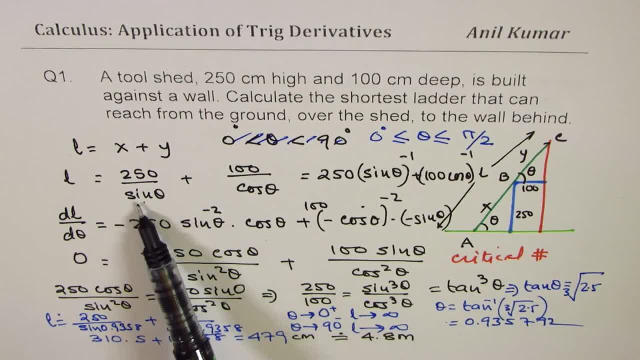 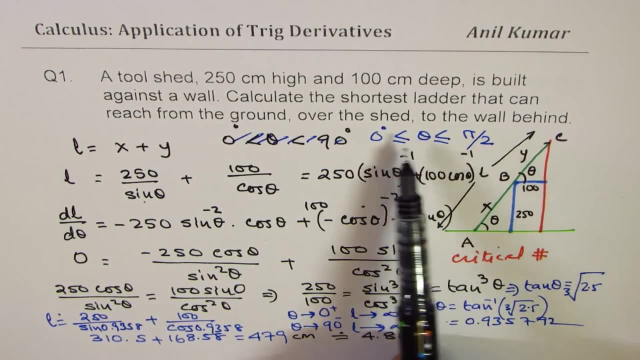 point nine, three, five, seven. substituted that value to find the length of the ladder: four point eight meters or four seventy nine centimeters. perfect. now it's important to understand that theta can be within zero to pi by two. I should say zero plus and less than pi by two when theta approaches zero. 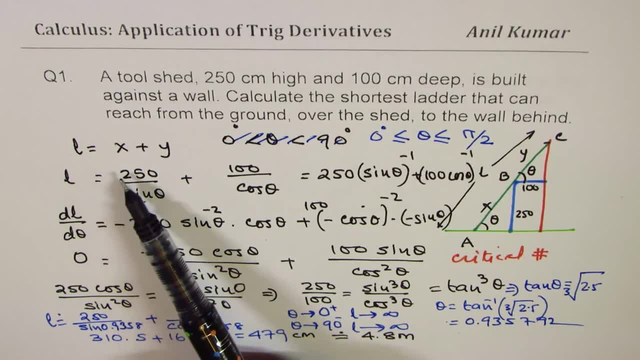 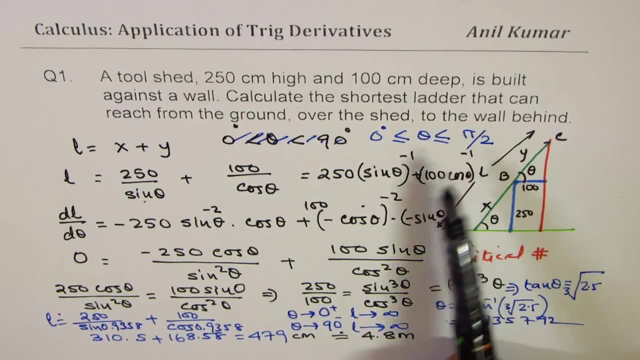 sine, theta approaches zero. so two fifty divided by zero will be infinitely large. but when theta approaches the other extreme value of pi by 2 cos, theta approaches zero. so in any case, anything in between will give us a minimum, do you understand? therefore, we know this is a minimum, right, and that is the. 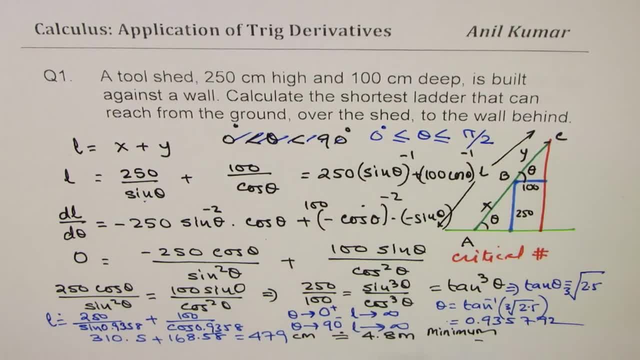 justification by testing endpoints. is it okay, since there is a closed interval? points: is it okay, since there is a closed interval? is it okay, since there is a closed interval, and, in fact, we might get great expectations? if, though, our minimum, low minimum, underestimated, there can be slim as much a good expectation what we can do. 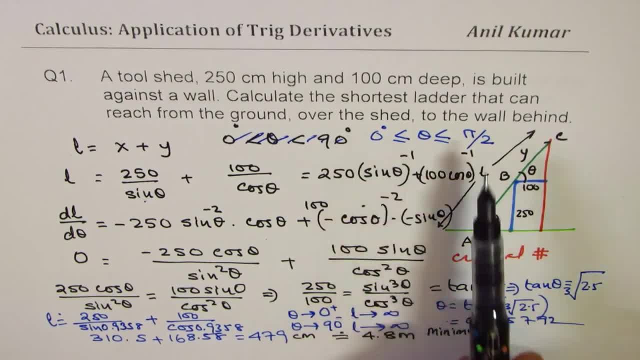 is you use a minimum or you give us? is it 20 plus a very large by two, and that is a true four, which is normally the minimum. we said so occasionally: two pi minus three, theta is between 0 to pi by 2. now let's move on to question number two. question number two. 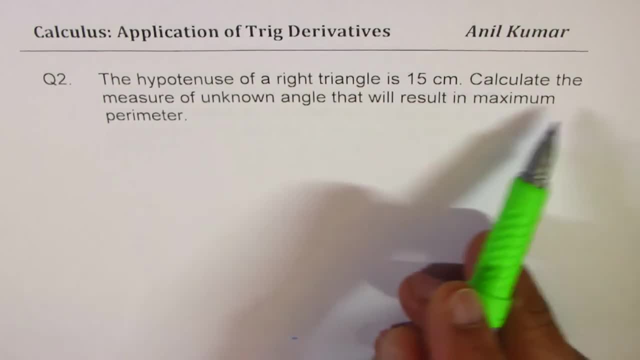 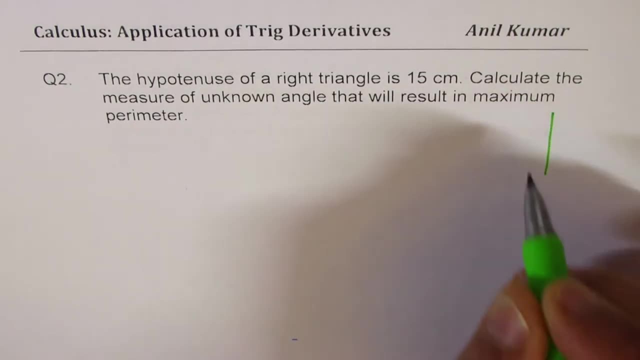 the hypotenuse of right triangle is 15 centimeters. calculate the measure of unknown angle. that will result in maximum perimeter. so let's sketch our triangle. this is a right triangle with hypotenuse as 15 centimeters. let the angle be theta, this side be x and the other side be y. 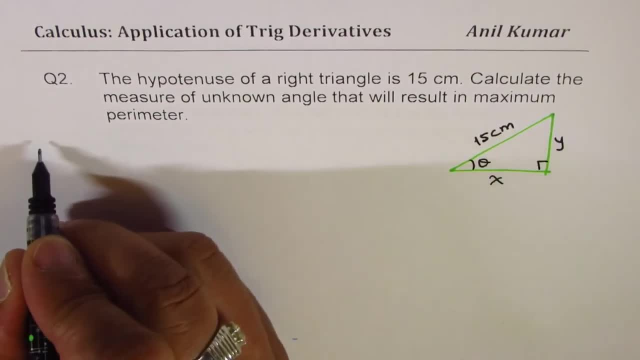 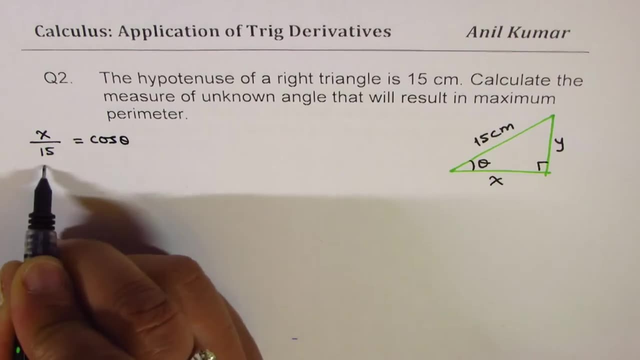 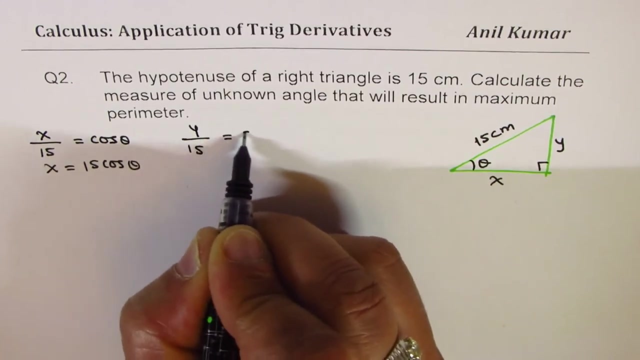 right. so that's the right triangle triangle. so from the triangle we know x over 15 is cos theta and that gives you x equals to 15 cos theta right. and we know y over 15 is sine theta, so we can write y equals to 15 sine theta. 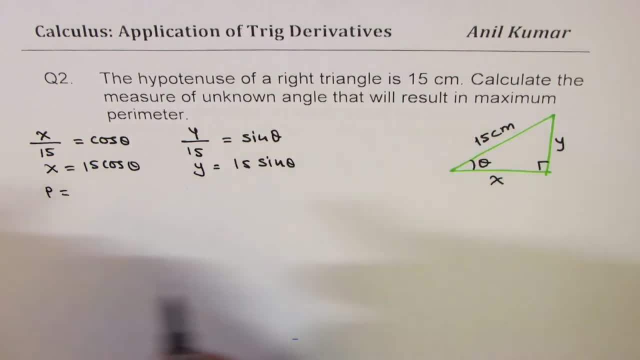 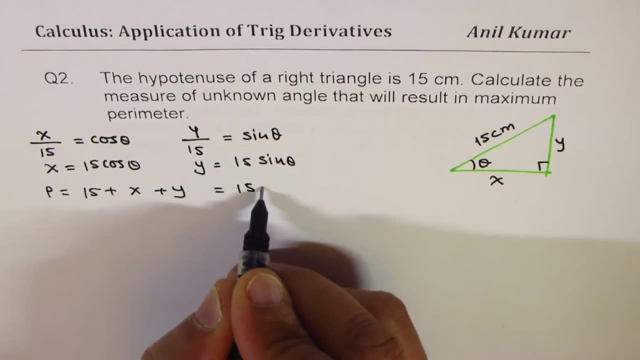 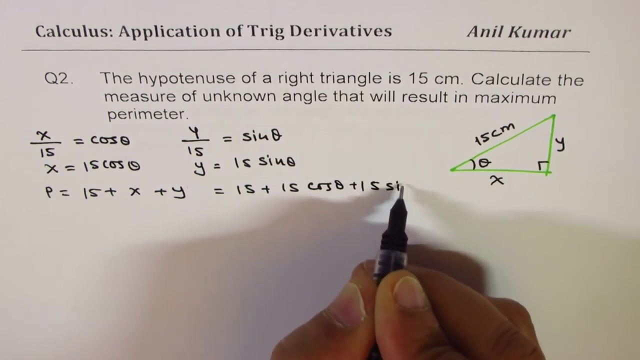 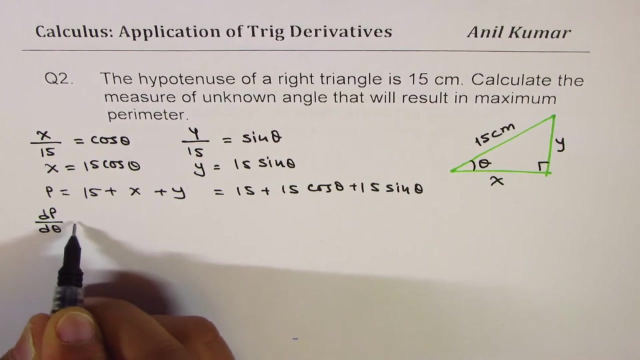 so what is perimeter? perimeter is sum of all three sides, which is 15 plus x plus y, and that could be written as 15 plus 15, cos theta plus 15 sine theta. clear. now, to maximize the perimeter will differentiate the perimeter with respect to theta. that constant will be 0. here we'll get 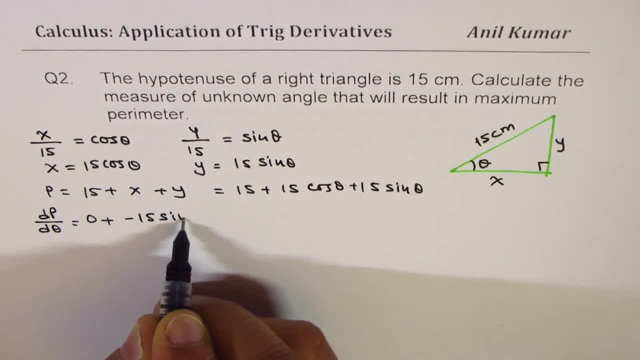 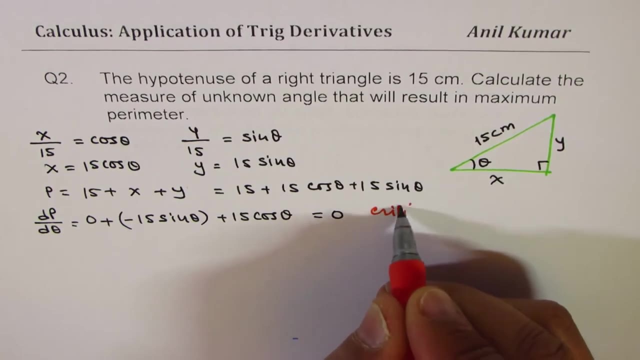 my minus 15 sine theta, and The derivative of sine theta is cos theta, so you get plus 15 cos theta. For critical number this is equal to 0, right? so this is 0 for critical number, And therefore we can now take it to the other side and say: 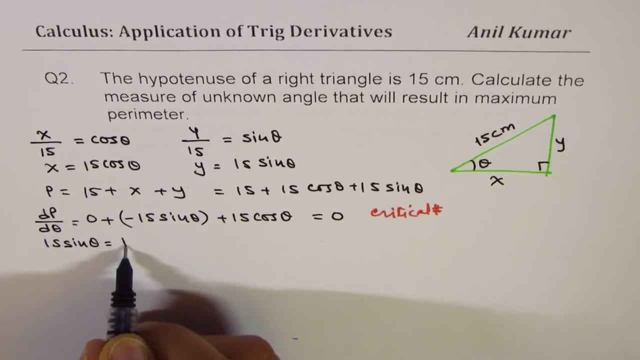 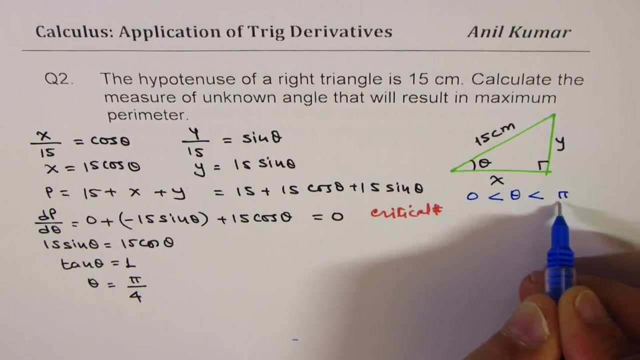 15 sine theta equals to 15. cos theta, or Dividing, we get tan. theta equals to 1, and This is when theta equals to pi by 4, right? so remember, in this particular case, We are taking theta which is in fact between 0 to pi by 2. 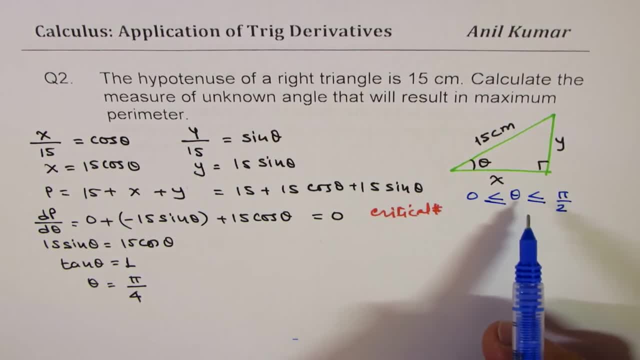 We'll write this as a closed interval. however, we know That if it is 0 will kind of get like this Right, so this will coincide with the adjacent side. Now you should remember one thing: that Cos theta is going to be. So anyway, let's figure out the dimensions also and see. with this we get maximum or minimum right. so first, 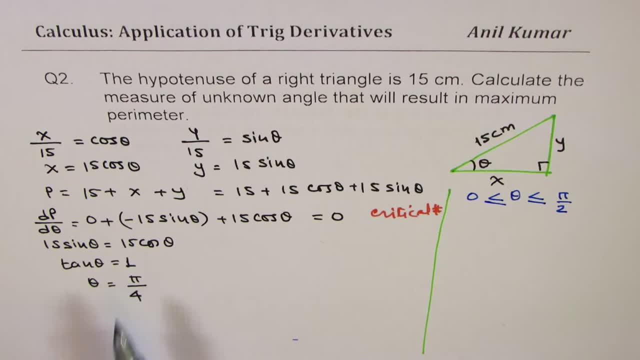 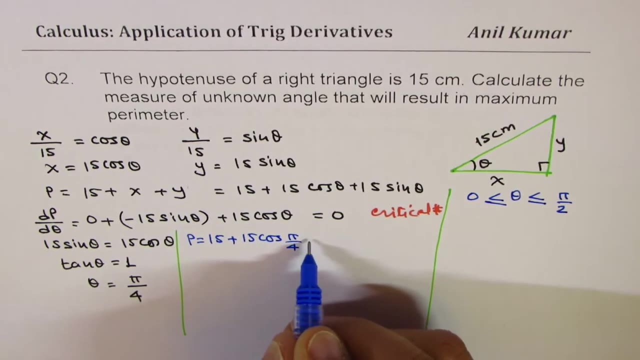 We got critical number as pi by 4. now if theta is pi by 4, in that case, What is the perimeter? let's find this out. So in that case perimeter will be 15 plus 15 cos pi by 4 plus 15 sine pi by 4, correct? 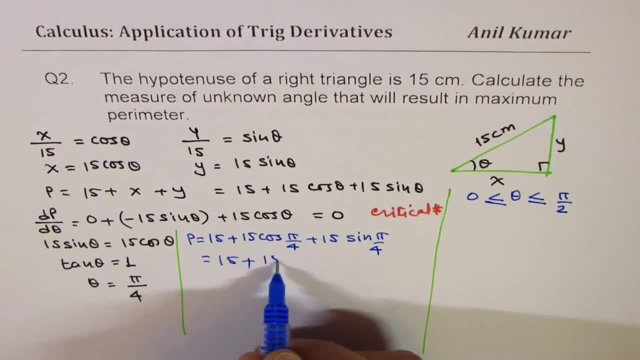 So that gives you 15 plus pi by 4 cos. pi by 4: 1 over square root 2 right, and This is also 1 over square root 2 right, so which is 15 over square root 2, So that gives you 15 plus. 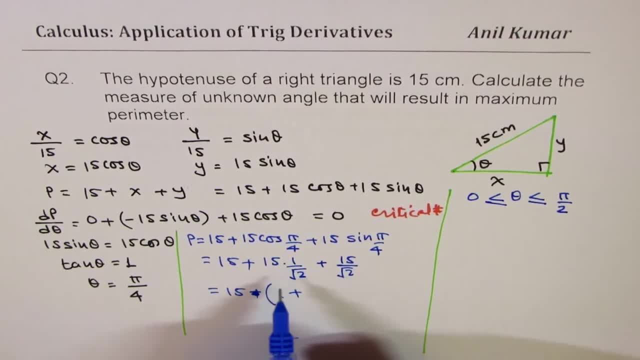 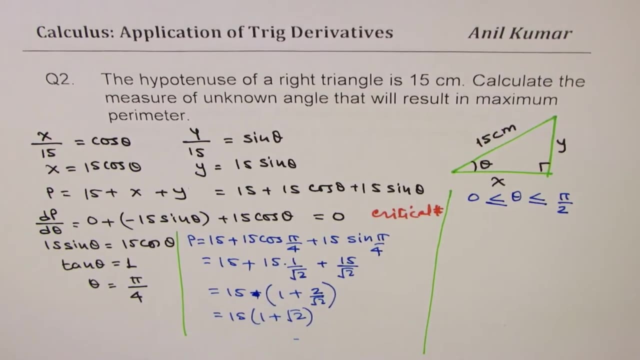 So if I take 15 common, I get one plus, and here I get 1 plus 1 as 2 over square root, 2, or We could write this as 15, 1 plus Square root. is it okay? so that becomes the parameter. so whatever is the length of hypotenuse times. 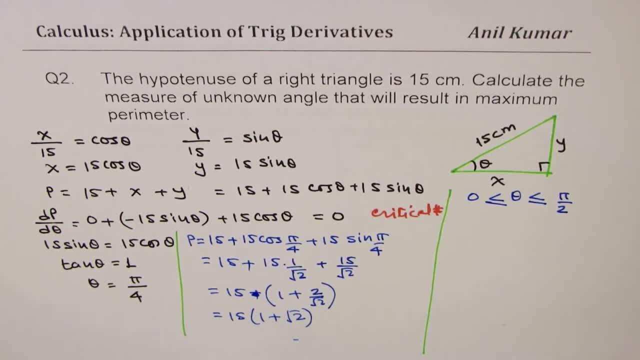 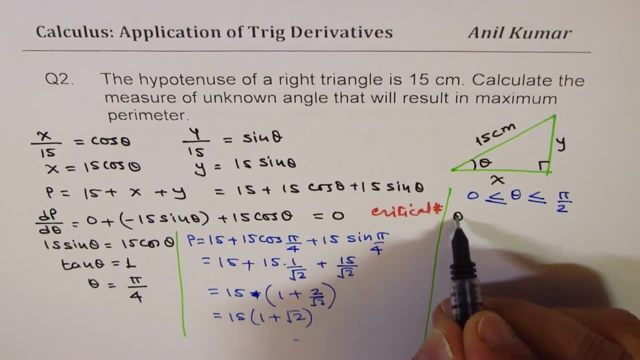 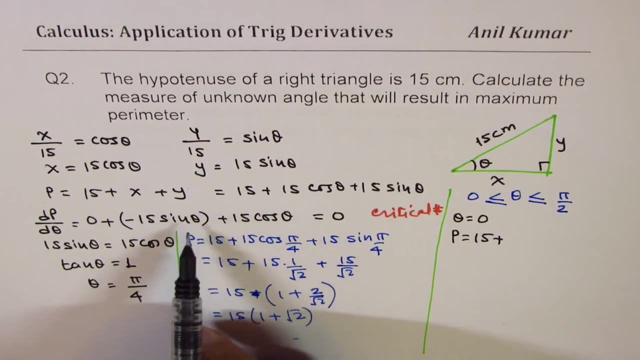 1 plus Square root 2. Now let us check if this is is the maximum or minimum right, because this is a critical number. so if theta equals to 0 radians, in that case p will be equals to 15 plus for theta 0. sine theta is 0, right? so we have 15. 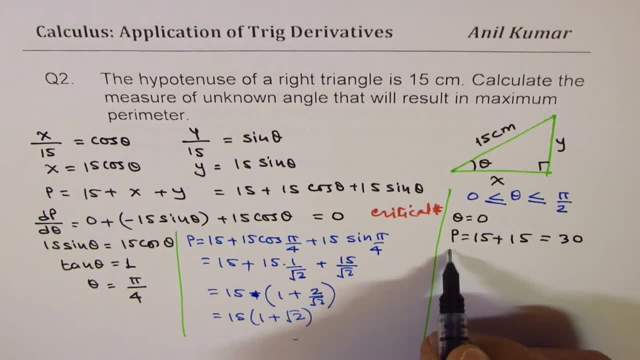 plus 15, which is 30, and if theta equals to pi by 2, in that case we know cos- theta equals to 0, so p equals to 15 plus this 15, right? so in either case we get 15 plus 15 as 30, but in this particular 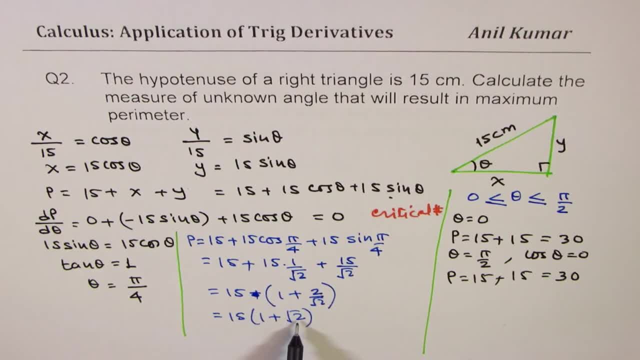 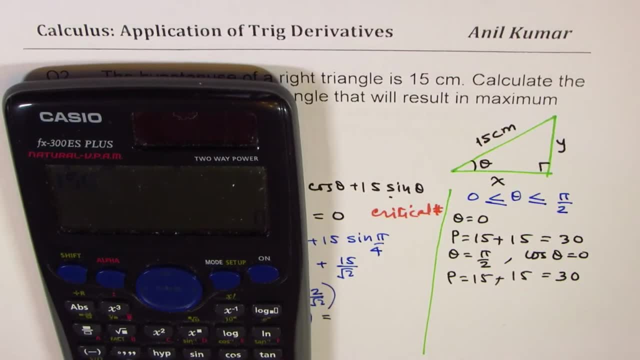 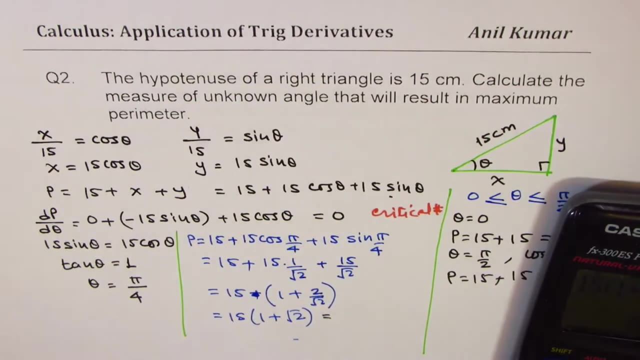 case, we know, square root 2 is more than 1, right? so in this case, what do we get? let's calculate: so we get 15 within brackets 1 plus square root 2. bracket close equals to 36.21. so we get 36. 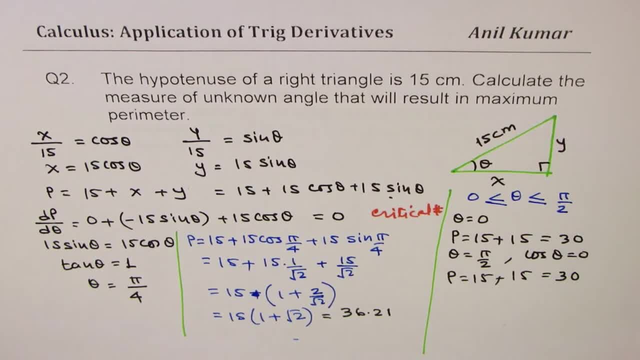 point 2: 1, units being centimeters right. so comparing the values, we know maximum parameter is equals to 36.21, but we need to only find find the unknown angle, that is, for angle, theta equals to pi by 4 radians, is it okay, radius? so that is how it will be solved. now let's take up. 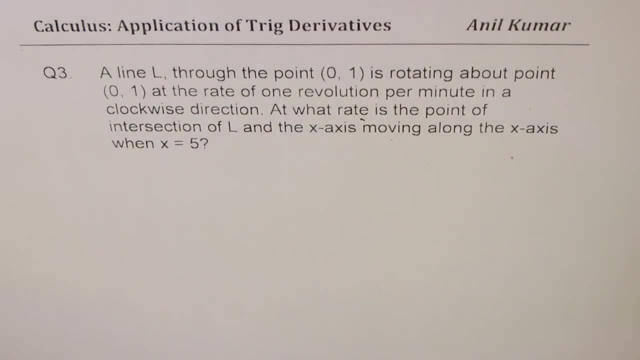 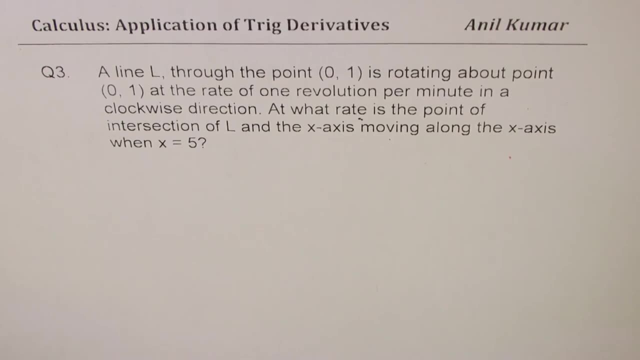 the other examples. i am anil kumar, sharing with you a very interesting question on rate of change: application of trigonometric functions. question number three: align l through 0.01 is rotating about 0.01 at the rate of one revolution per minute in clockwise direction. at what rate is? 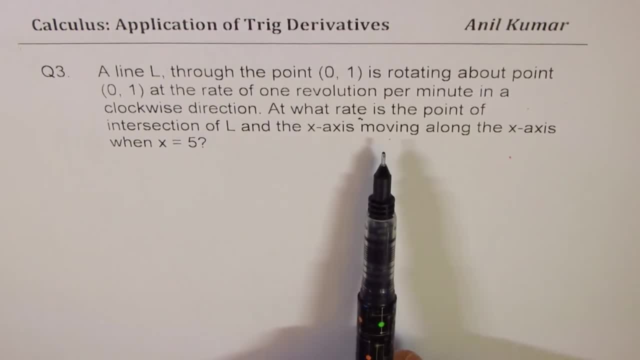 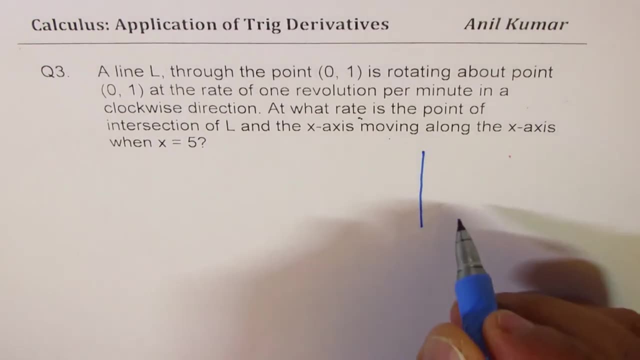 the point of intersection of l and the x-axis, moving along the x-axis when x equals to 5. so let's sketch this to understand the situation and then we'll figure it out. so we have a line kind of like this, which is rotating about a point: 0, 1. so 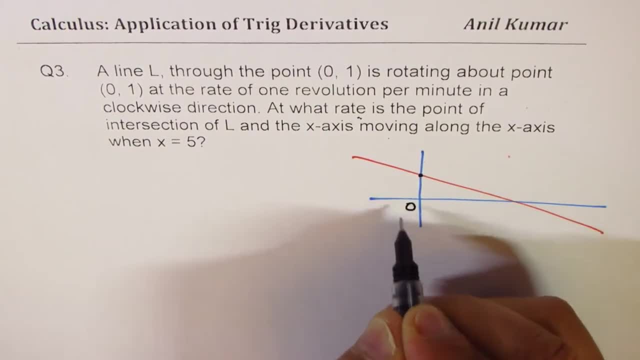 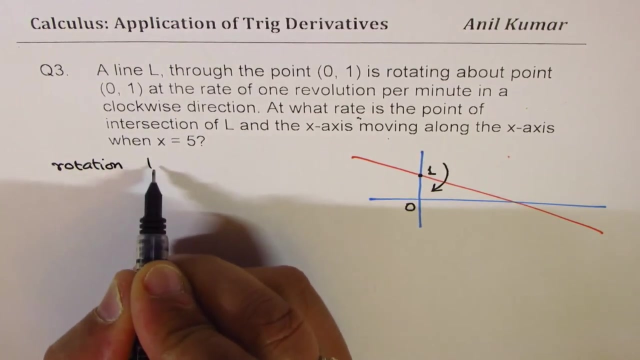 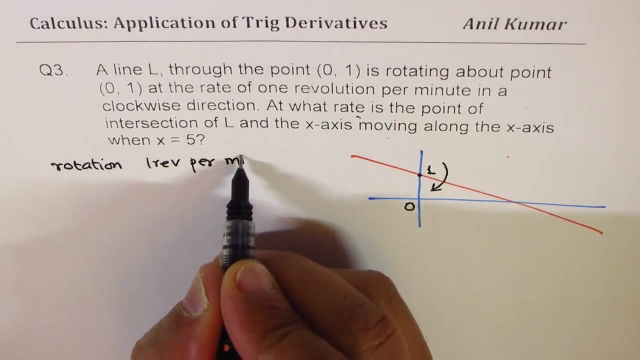 that's your y intercept. this is the point: 0, 1, right. so 0, 1. so when it rotates, it's rotating in clockwise direction. it's rotating in clockwise direction, so the rotation is given to us as one revolution per minute. now, this will be considered negative. 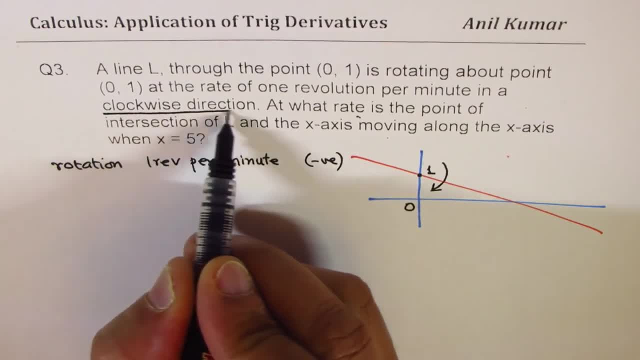 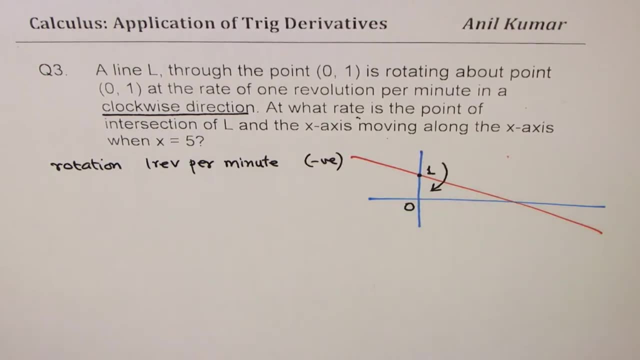 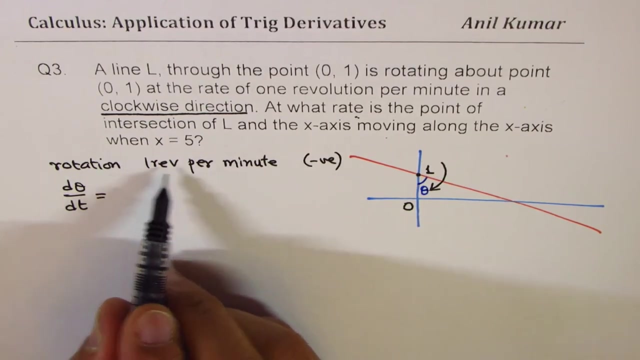 since it is clockwise, right, since it is clockwise, is that clear? so one revolution per minute is the rate of change of angle. so if i say that this angle here is theta, let's say: let's keep this angle is theta. in that case, what we are saying is that d, theta, dt is equal to one. revolution means two pi. so i 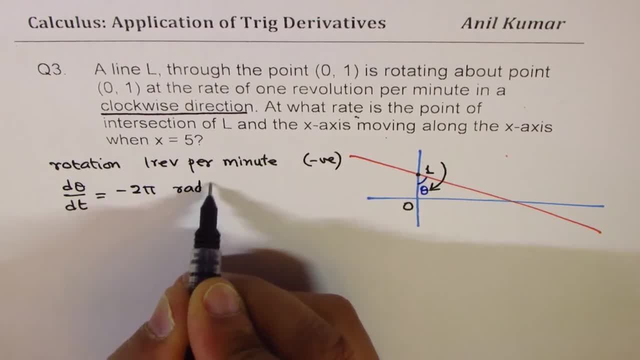 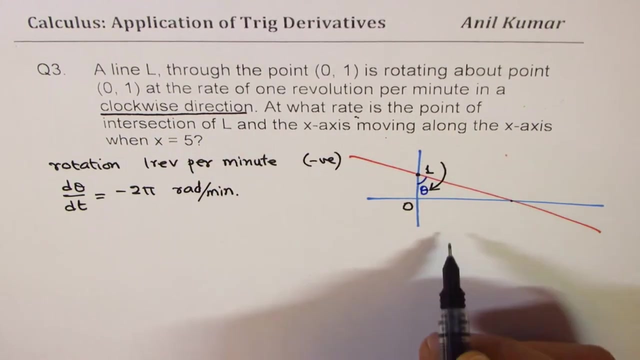 can write this as minus two pi radians per minute, correct, so that becomes d theta dt. now we want to find at what rate is the point on of the l and the xx. let's say this is the x intercept, so this point is moving. let's call this point as a when x is five. when, when this. 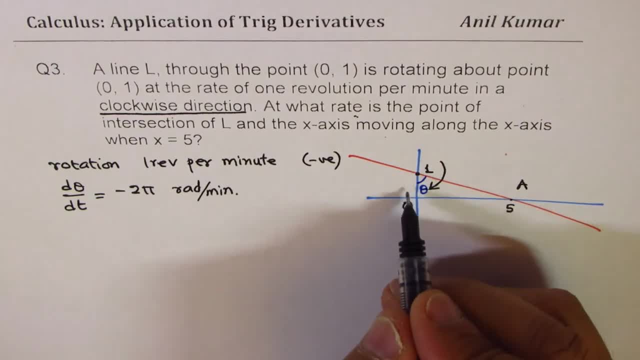 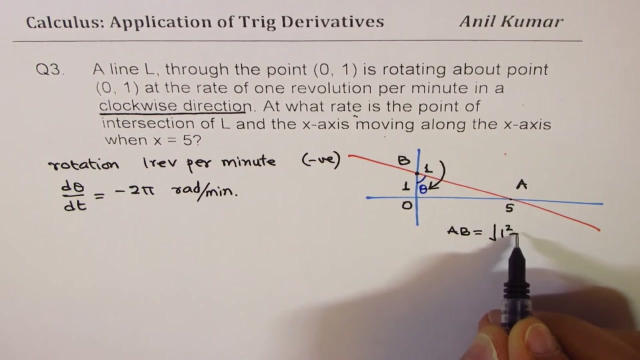 x is five. that is what it is when this is fixed at one. let's also calculate. let's call this point as b. so what is a b equals to? let's write down here: a b will be square root of one square plus five square, correct you? 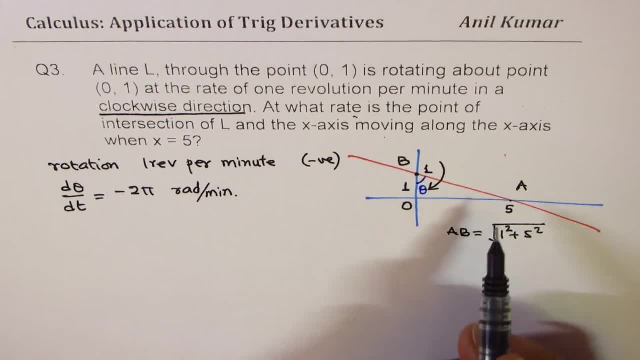 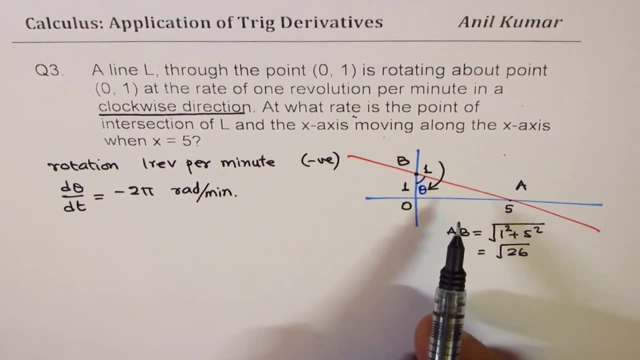 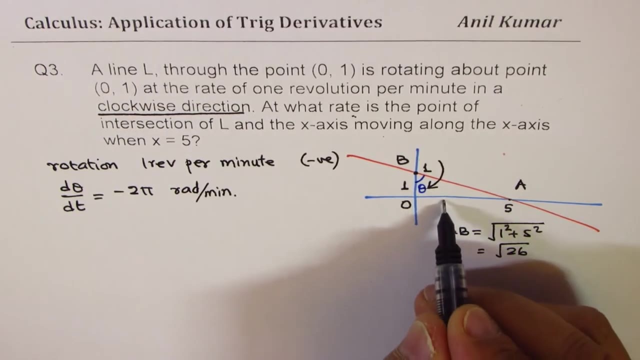 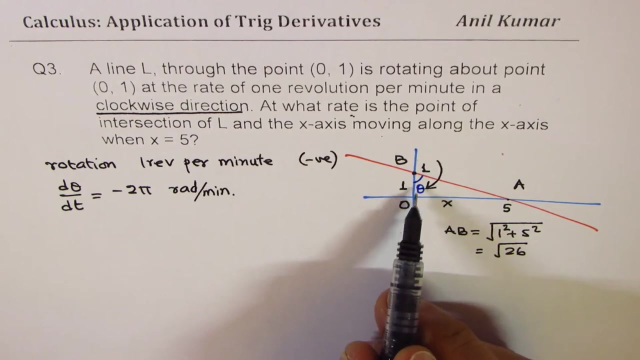 that is a b hypotenuse, okay, so, so, which is square root of 26? okay, now we can relate. let's say: this is x any time, right? if this is x? in that case, how is x related with theta and one, so that becomes the opposite side, correct? 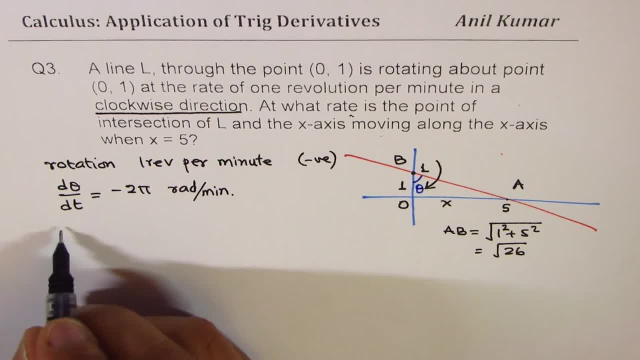 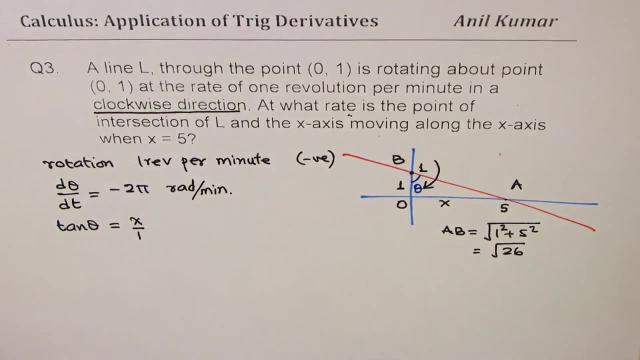 so that is the opposite side. so we can say: tan theta is equal to x over one, or x, is it okay? x over one. we can say that now let's differentiate both sides with, with t, right? so let's differentiate with respect to time. so if you do that, you get. 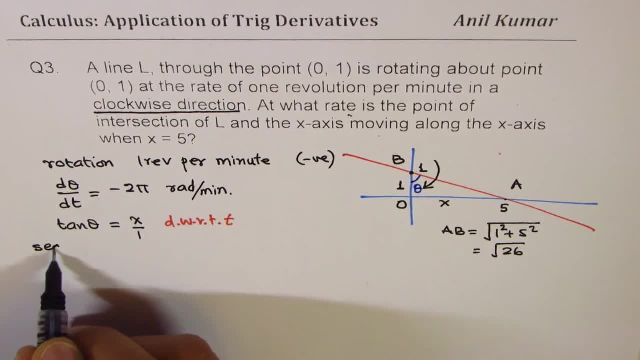 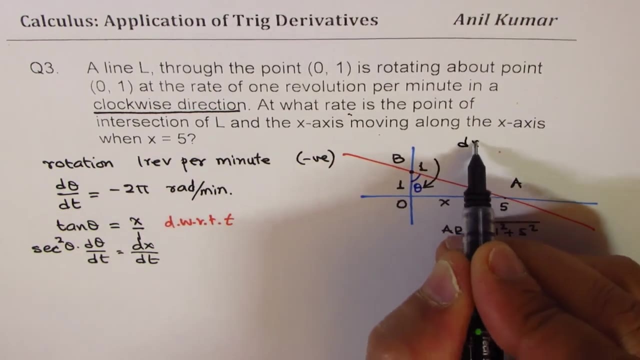 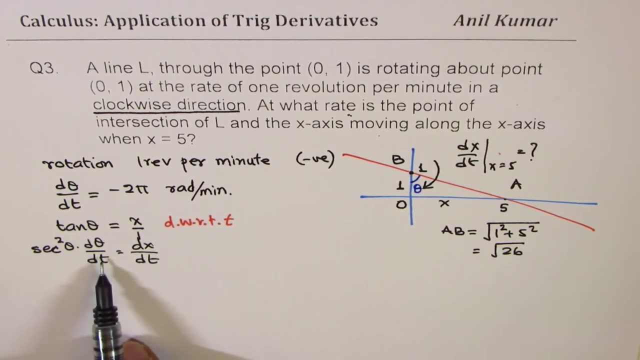 a secant square: theta d theta dt of x. sorry, d theta dt is aurious to that, so we'll available. oh, but b is the favourite set, right, okay? so how do I calculate that b? this is what we're doing in our equation. so d theta is equal to miggs, or d x equals ht. this is an infinite concept. then we generate all the a, which is equal to the antegram of our equation. we have two to the power under point 5, 0, which is equal to 0, l equals to dx dt, correct? and we actually need to find d x dt when x is five. that's the whole idea, right? so we need to find dx dt when x equals 5. this is what we need to calculate. so that is what we know a reality, and it is. we know d theta. dt is a symmetric minus 2pi and for the given angle, theta. what is secant theta? 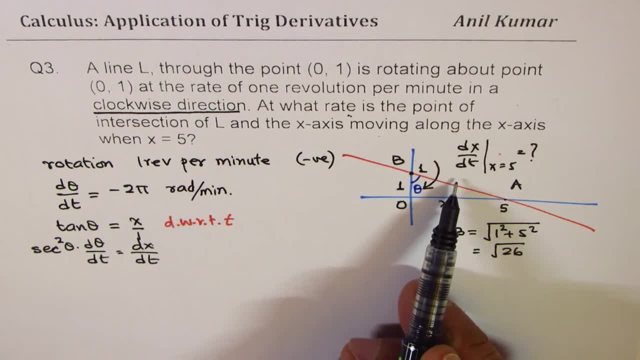 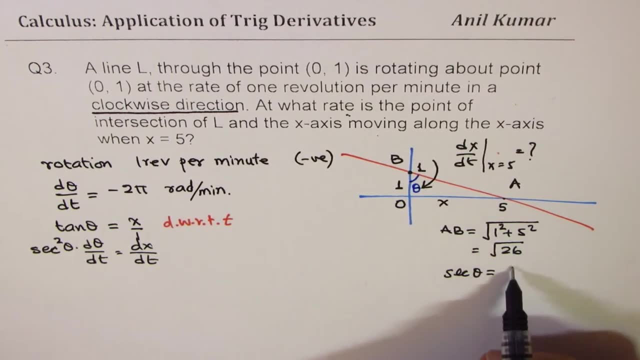 well, secant theta will be hypotenuse over adjacent side. so in this case secant theta will be hypotenuse square root 26 right over over one. so secant theta, square root 26. so we know this. we are going to substitute this here. so, substituting, we get square root of 26. 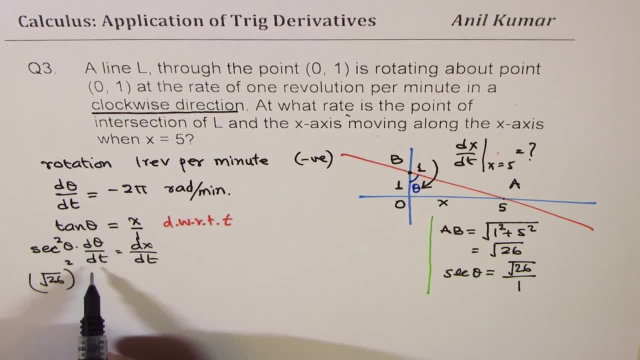 whole square d theta. dt is known to us as minus 2 pi, which is minus 2 pi is equals to dx, dt, correct? so? so that is what it is now. we can just multiply this and that is 26, right? so we get minus 52 pi equals to: 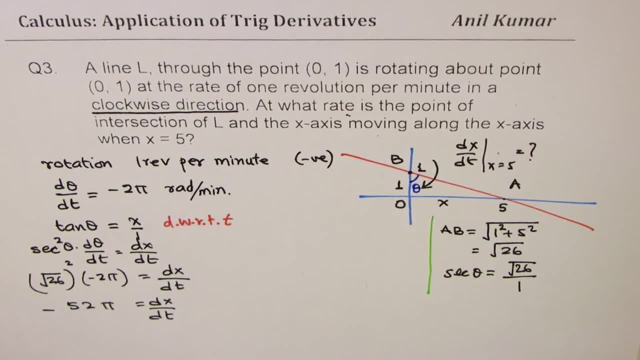 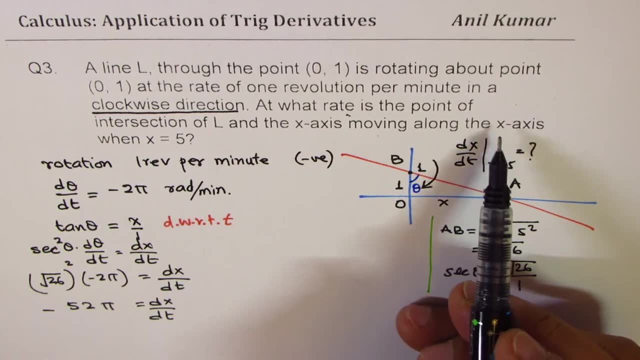 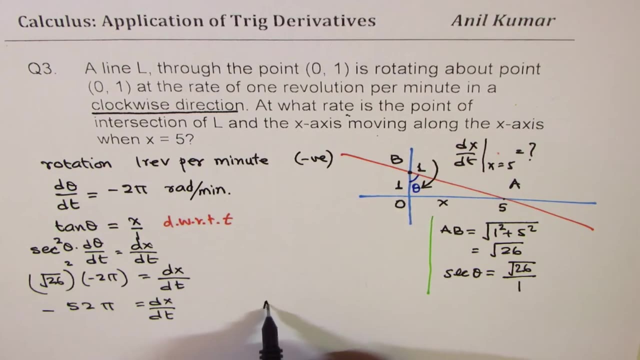 26 dx dt does make sense, right. so that is what it is. the units will be. well, we are not given any units along this side per minute, so okay, so whatever units, units per minute, so we get our answer, which is the rate of change at this instance of time will be. it is decreasing, right. 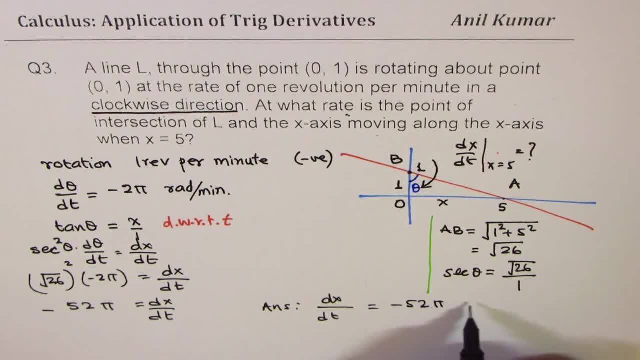 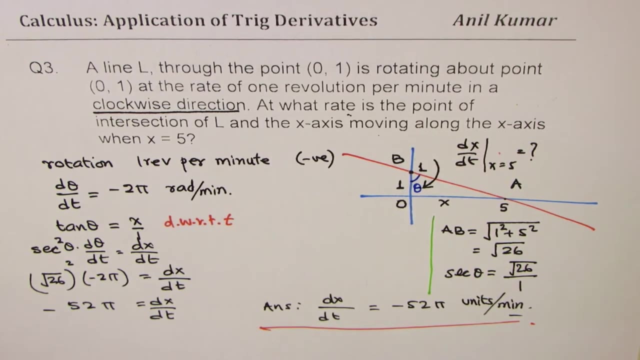 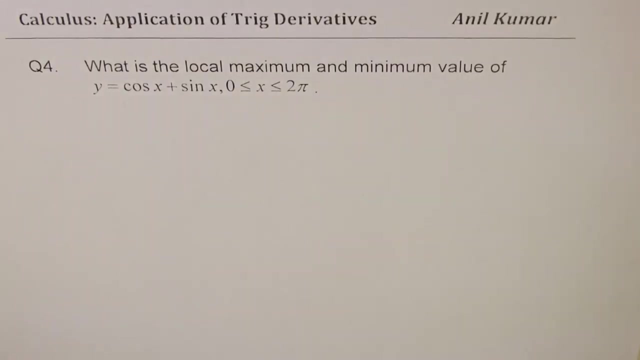 that negative means decreasing minus 52 pi units per minute. okay, so that is how we are going to solve it. i hope it is absolutely clear. feel free to write your comments and share your views. okay, now let's move on and take the last question, which is question number four. now it says: what is the local maximum and minimum value for y equals to: 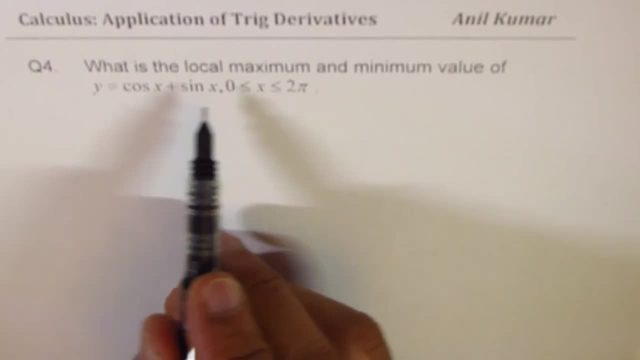 sine cos x plus sine x when x is between zero to two. so let's draw still question where x is between 0 pi and it's between 0 to two pi. so it's a simpler. look. I want you to pause the video. answer this question. look into my suggestions. we are looking for local maximum and minimum that is, from y equals to cos x plus sine x. 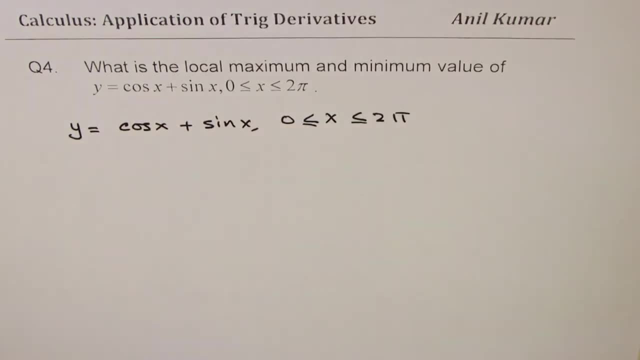 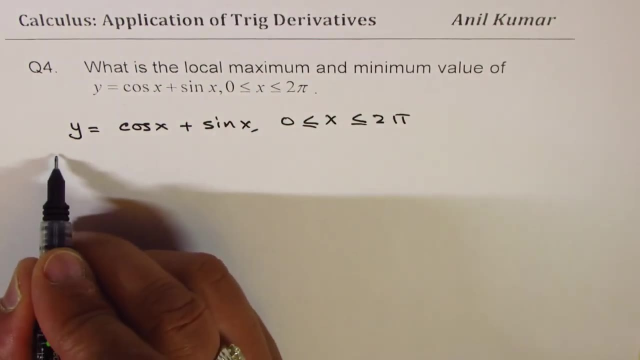 cosine assigned is two pi, where I guess f is between zero to two pi. I like you to pause the video, answer this question and go to my suggestion. we are looking for a correct answer. local maximum minimum. so we find the derivatives. so we say dy, dx is equals. 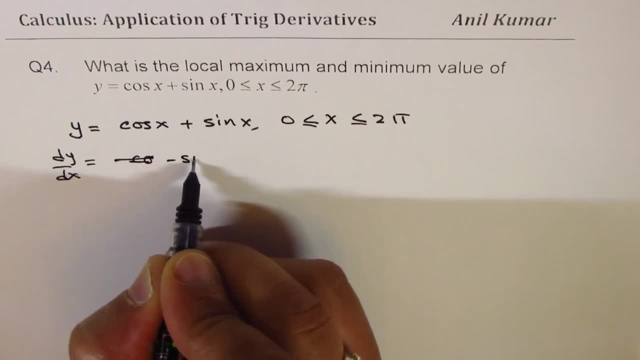 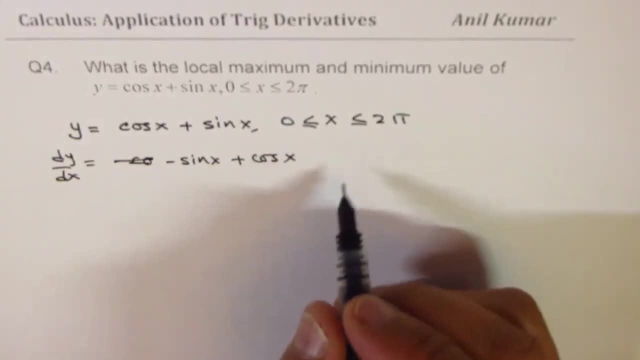 to minus wine, plus the derivative which is momentos in the therefore弟 él, based on the sides xc frontburners is equal to minus. where is 0 tie in minus sine x plus cos x. the derivatives right Now for maximum or minimum. 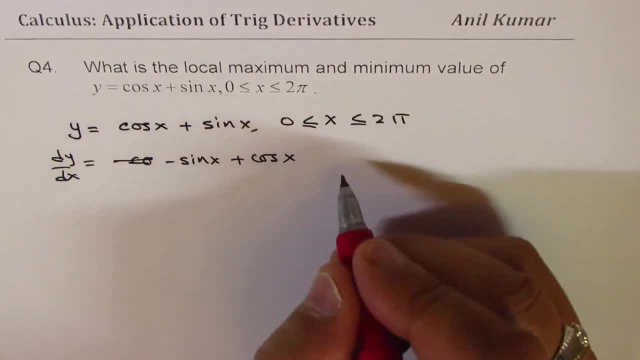 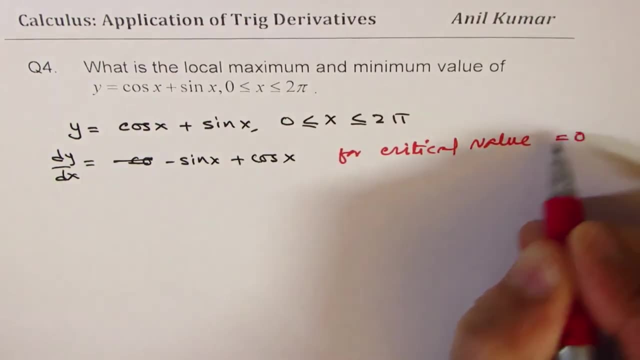 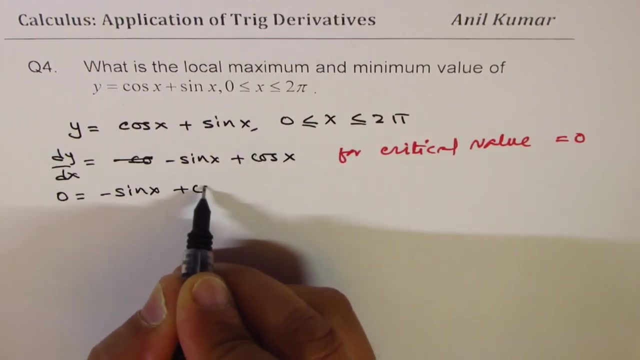 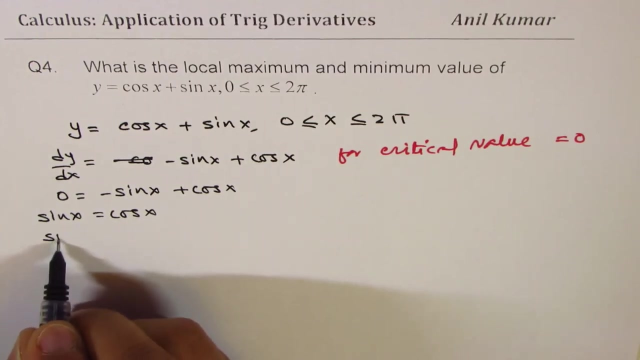 we say the critical number, this should be 0, right? So for critical value, this should be equal to 0. So let's say 0 equals to minus sine x plus cos x. So sine x will be equals to cos x. or when you divide, you get sine x divided by cos x. 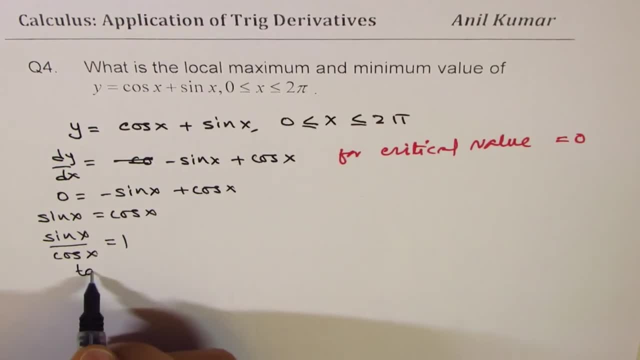 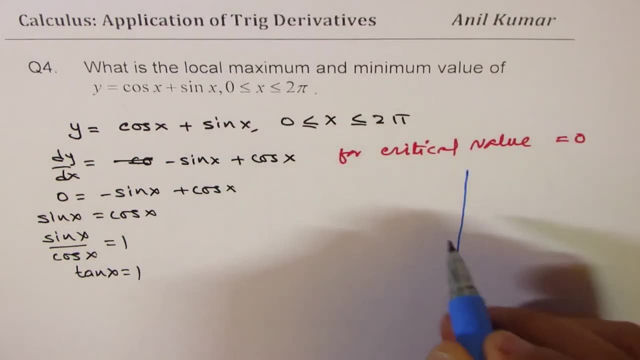 equals to 1.. So that gives you tan x equals to 1. and between this, when is tan x 1?? Positive 1, when either you are in quadrant 1 or in quadrant 3, right The angle being pi by 4,. 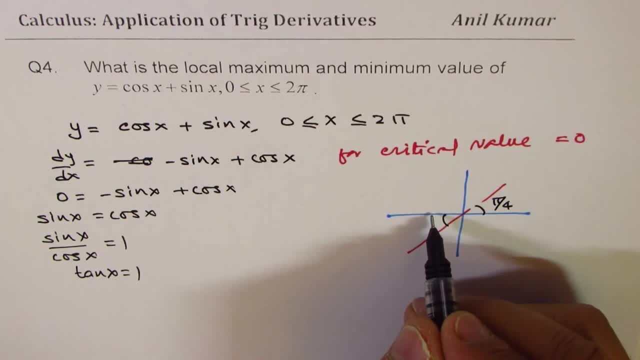 right. So this becomes 1, 2, I mean 1 pi by 4, 2, pi by 4, 3, pi by 4, 4, pi by 4, 5 pi by 4 or this right. 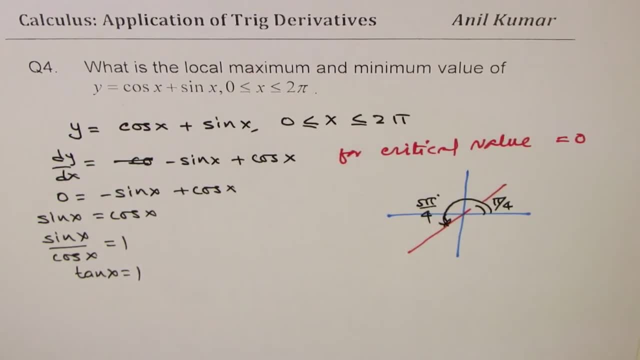 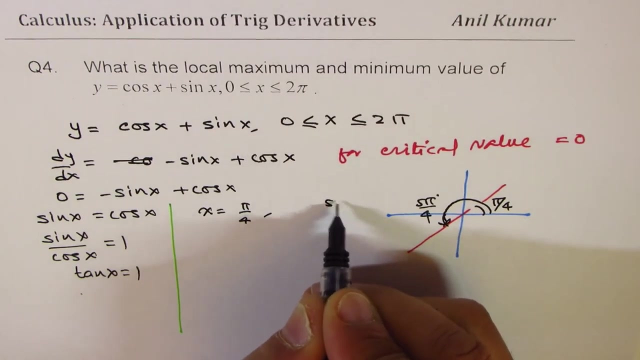 5 pi by 4, correct, So those are the angles. Okay, So we get from here. let's write down here 2 values: x equals to pi by 4 and 5 pi by 4.. Now both these values will give us two different answers. Let's calculate the value of y. 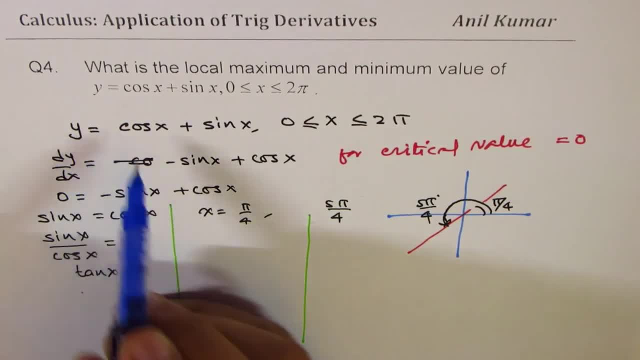 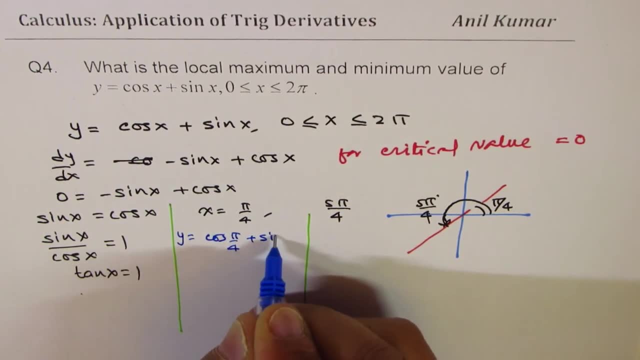 That should be simpler, So we'll just calculate y. So y equals to cos pi by 4 plus sine pi by 4, and also y equals to cos 5 pi by 4 plus sine 5 pi by 4.. So this is 1 over square root 2 plus 1 over square root 2, and this value is negative. of this, 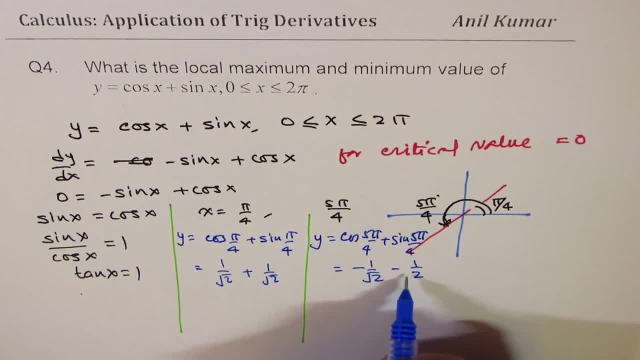 right. Negative 1 over square root 2, negative 1 over square root 2, okay, So that gives you the value as 2 over square root 2 or just square root 2.. Positive, and this will give you negative square. 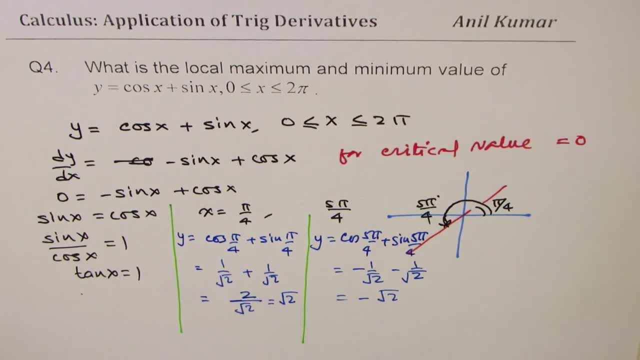 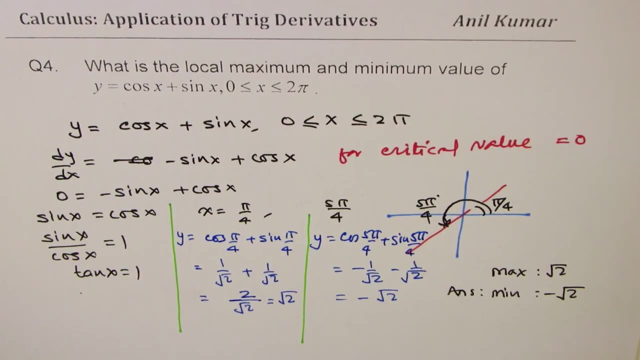 root 2.. Perfect, So we get our maximum and minimum values. So the answer here is: maximum is square root 2 and minimum is minus square root 2.. Does make sense, right? So that is how you could actually solve this question. With this, we come to an end on our four examples. 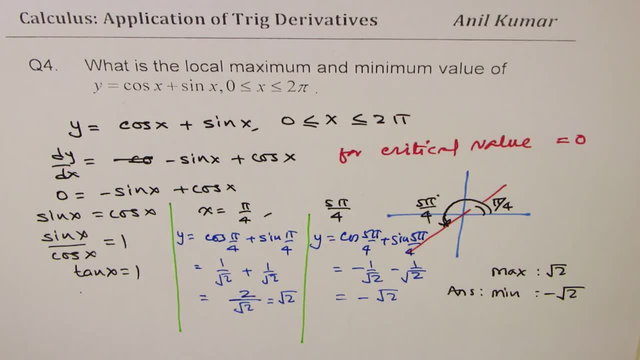 which we took for application of trigonometric derivatives. There are many more in my videos. I'll provide you with some links. Hopefully this gives you a fairly good idea about how to apply learnings and solve such questions. Feel free to write your comments. share your views.